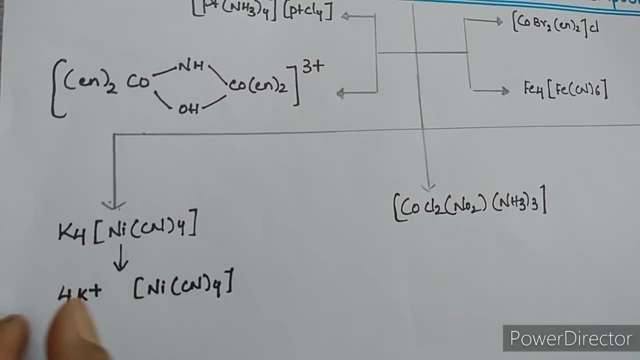 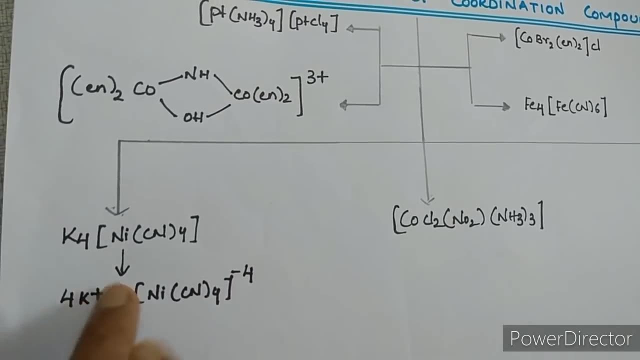 4 into plus 1.. So plus 4 is the charge on this cationic part. So to balance that, the charge will be down to 1 in terms of και to be subtracted by 2, It gets added this way will be 1. 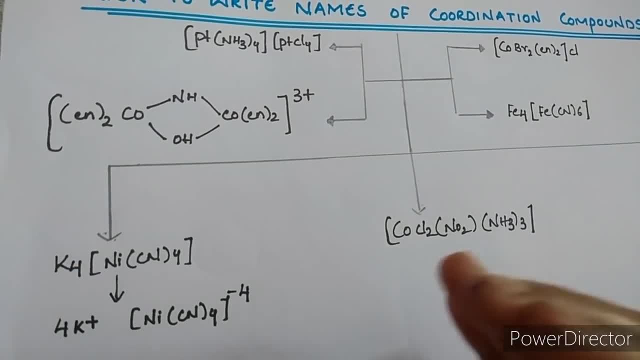 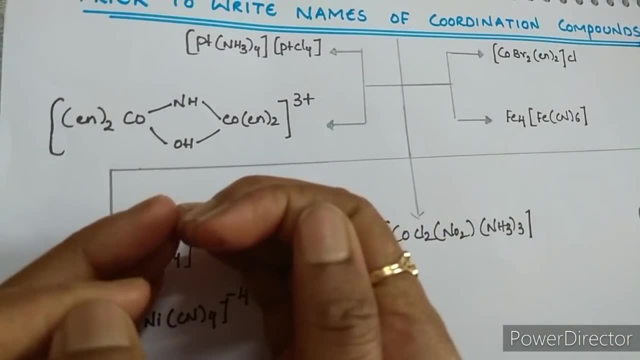 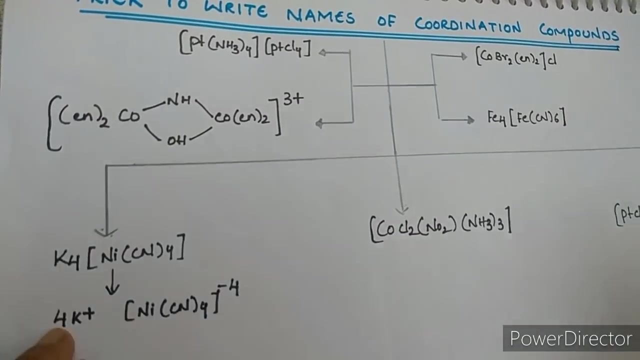 Ne, You will get as much as C4NICN4, so this is equal to half. so your D is the charge related to the charge, plus minus 4 would have become C2, which would be the charge right. Please watch the video till end so that you can understand what you are going to do. 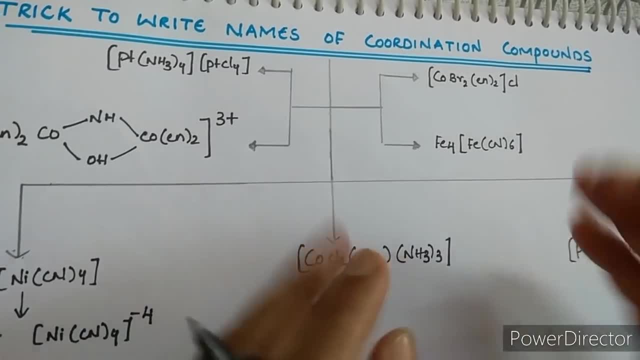 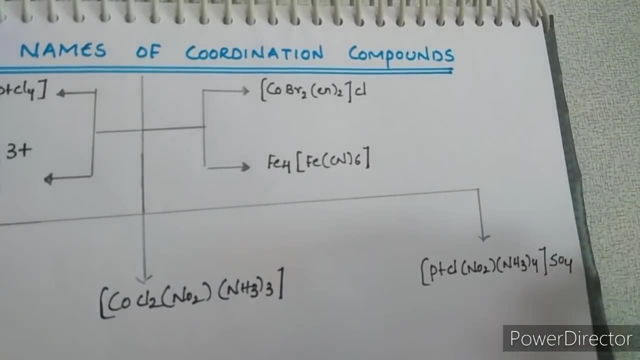 Let's provide all limits. Okay, So you need to C4O4C2.. one coordination sphere here, the ions which are present outside the coordination sphere, is this one, a sulfate ion, and this is inside. this is the coordination sphere. so first dissociate, like that. it will dissociate into ions. no, whatever there inside the coordination sphere it won't dissociate into ions. so here it won't dissociate any further ions. so the charge will be zero if it dissociate. like this: here it got negative charge and if it dissociate we get pt, cl no2 and nh3 4 it dissociating. 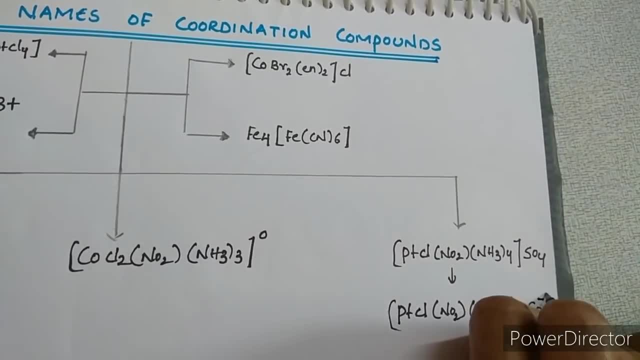 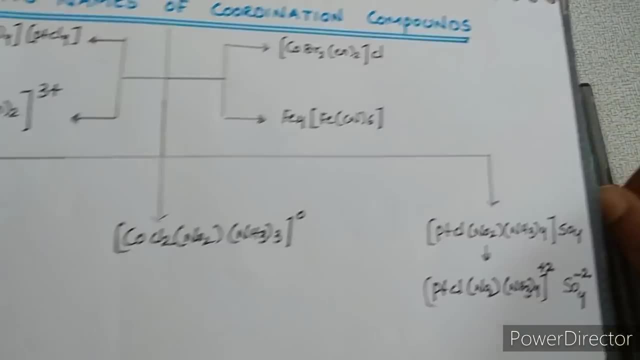 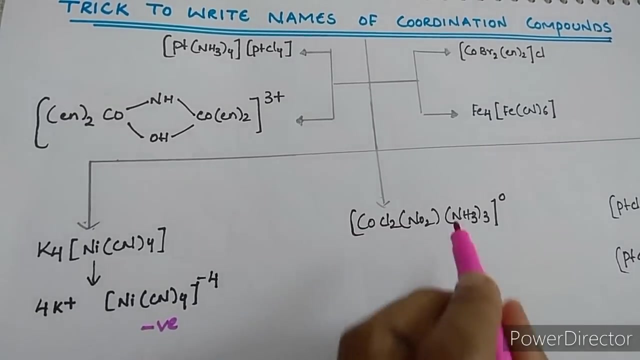 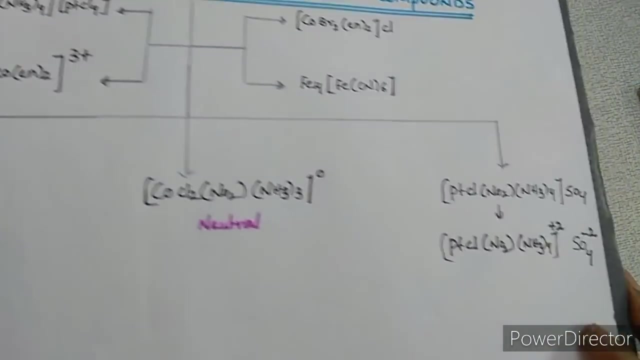 like this and so4 sulfate, it will be having minus 2 charge. if it gets minus 2, then obviously what is the charge on this? plus 2? got it? now observe clearly: this is the coordination sphere which is having a negative charge and this is a coordination sphere not having any charge. this is neutral coordination, complex and this 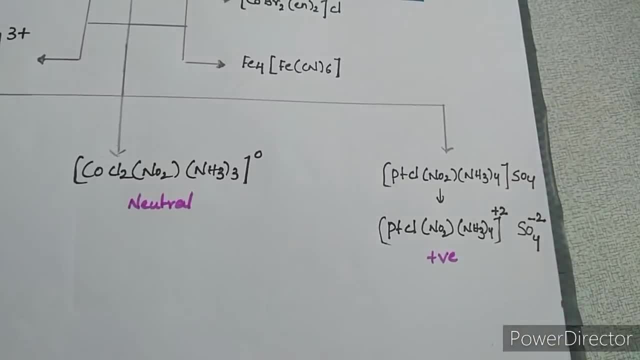 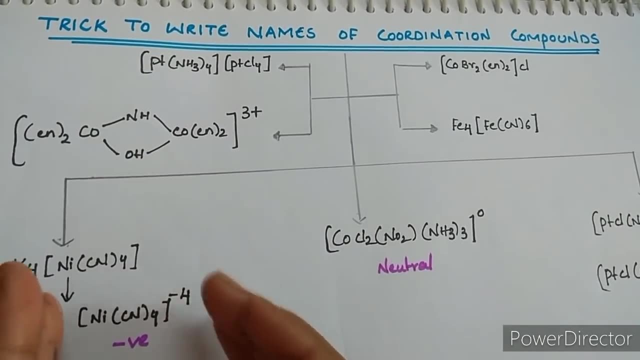 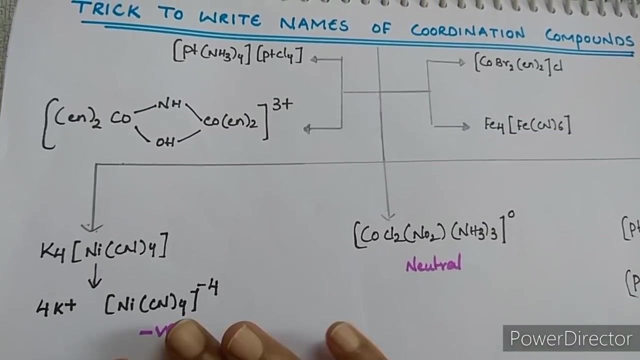 is a complex which is having a positive charge on it. so this is a three. i am going to classify this coordination compounds here into three. one is a complex with the negative, one is a neutral, another one is what positive. and one more thing, important point is here. i took the example of 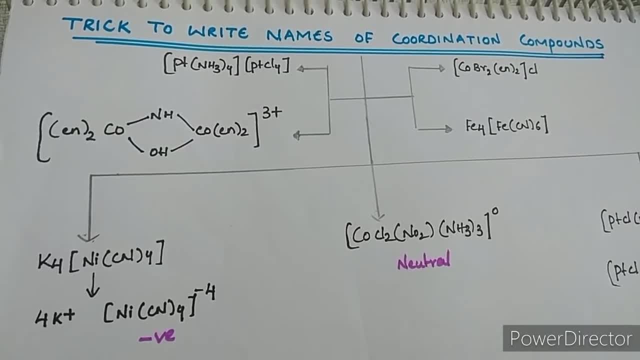 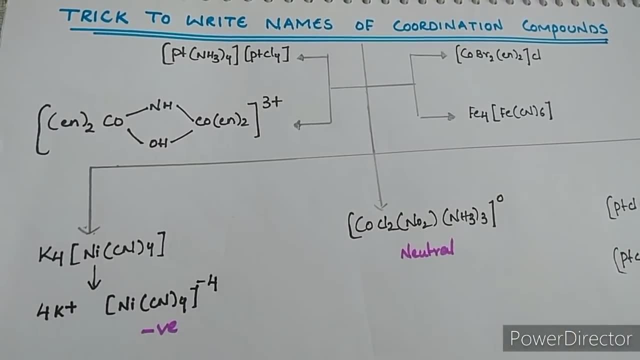 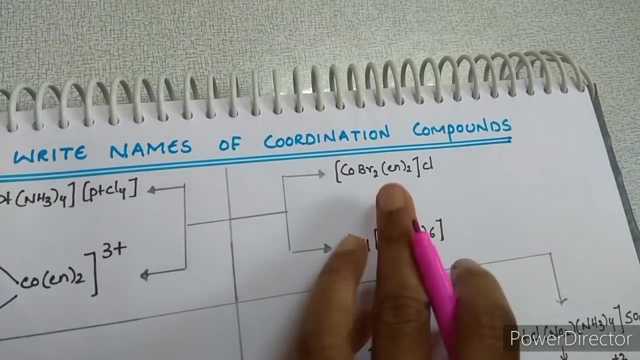 all monodentate ligands. ligand is the. what is the ligand, which is a molecule, donates a pair of electrons. here it donates only one pair of electrons, so it is called as a monodentate ligand, and this is the case where bidentate ligand is there. so i am going to discuss about bidentate. 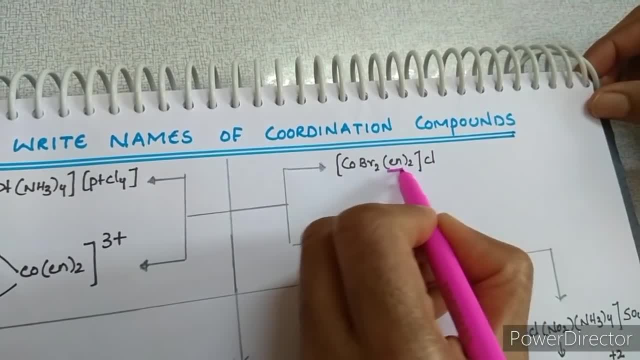 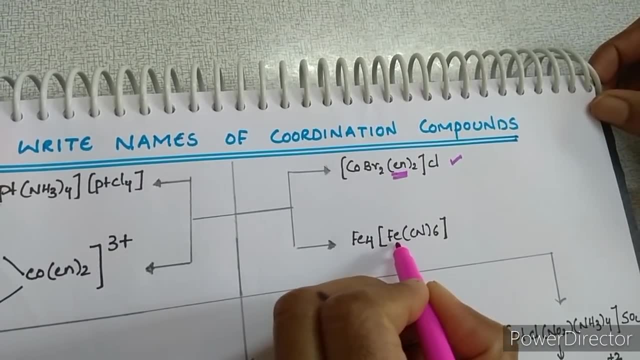 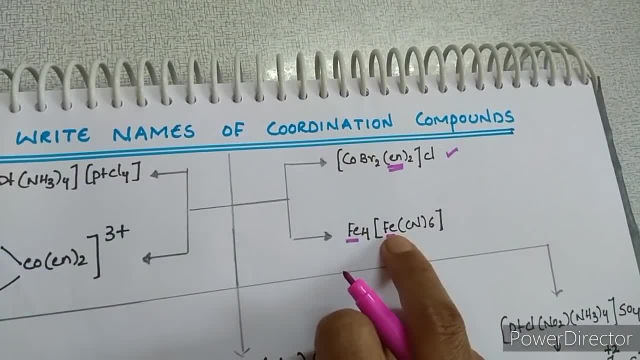 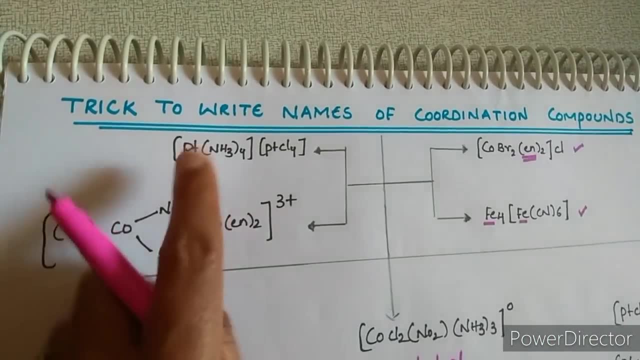 this is the one where you can see that. this is the one where you can see that. this is the one where two, two metals are there. one is there inside the sphere, same metal there outside the sphere- for this the way of naming will be different, clear- and here two metal atoms are there two. 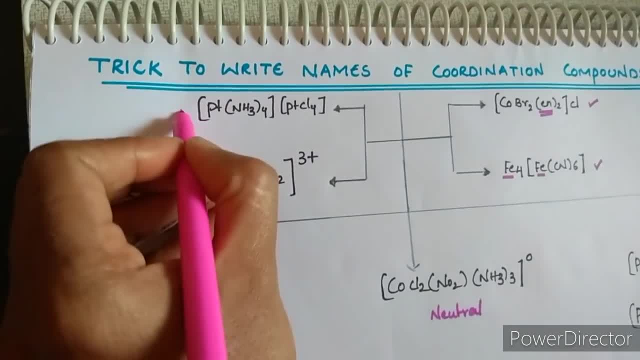 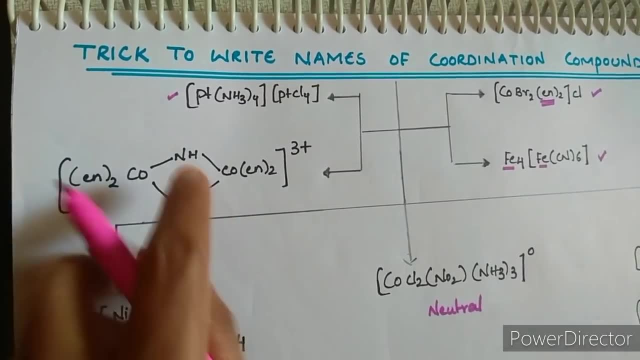 coordination complexes are there two complexes. for this the naming is different. and here bridged ligands is there. this is one bridge. this is one bridge. what is a bridge? the ligand which connects two metal, metal atoms is a bridged ligand. so in this case, uh, naming is 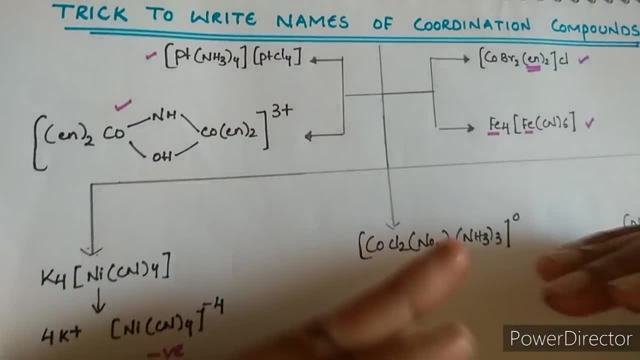 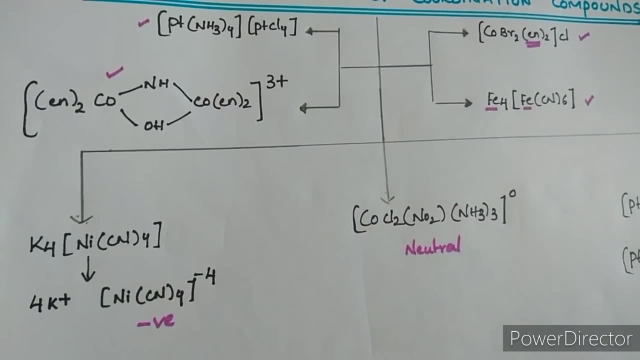 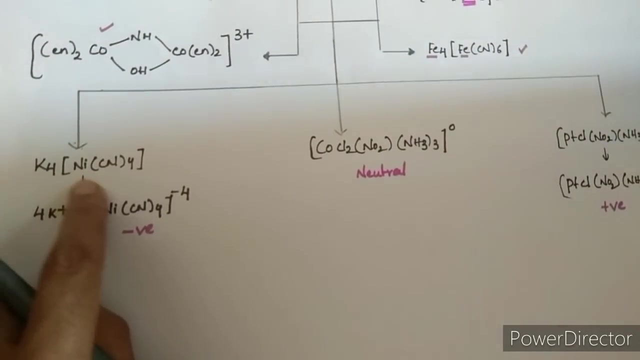 little different. so first follow the basics and the rules which i am going to discuss here. then it will be useful for you to follow the next sequence. definitely, i am going to do all this in very less time. now let us take this example: k4 ni cn4. what is that students? k4 ni cn4. 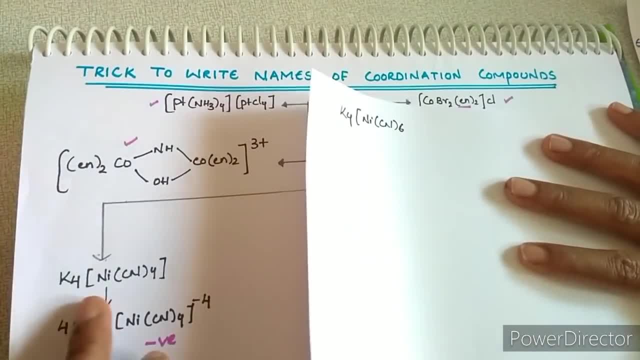 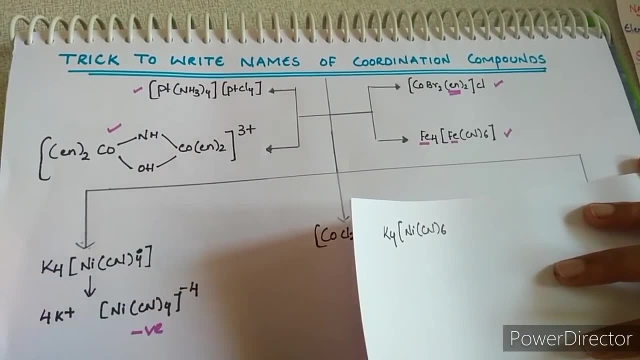 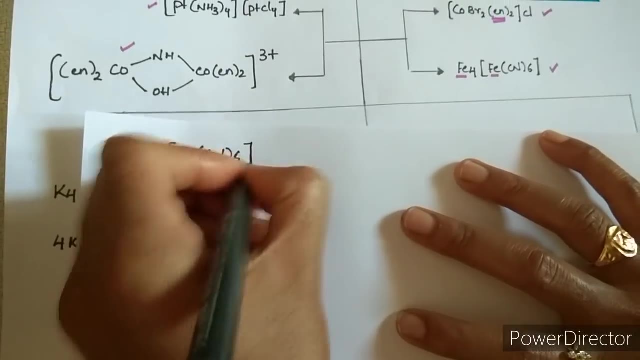 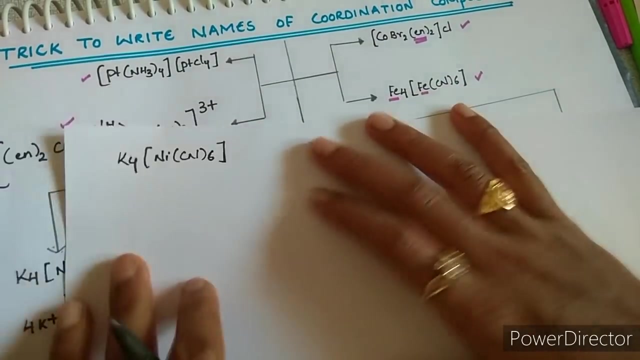 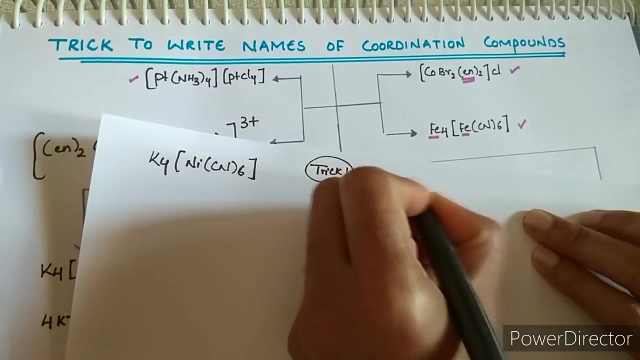 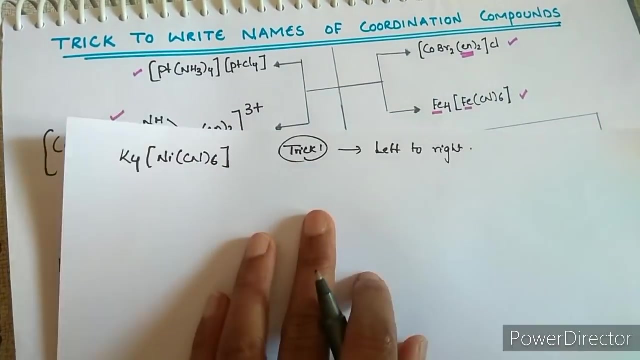 cn, k4, ni, cn6, cn6. see here, this is six. okay, this is six. this is the complex. keep it in mind, this is the coordination sphere which is getting negative charge. i will tell you how to do it always. point number one is keep it in mind that write the naming from left to right, left to right, so when you have to do left to right. 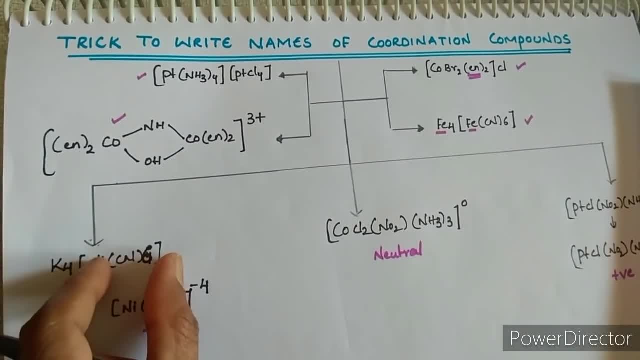 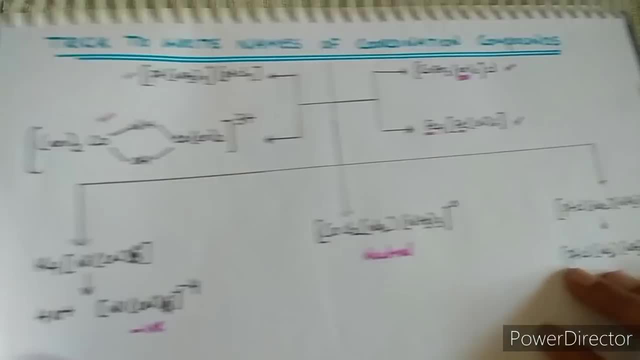 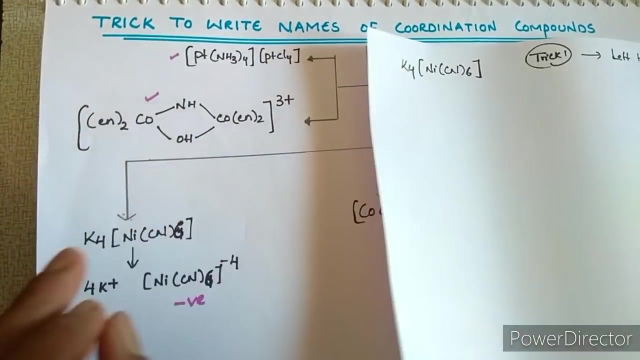 means here first potassium you should name and you should name the coordination complex here. there is no left here, nothing is there. so directly you have to name the coordination complex here first. you should name coordination complex, then the outer part. so always you have to name first from. 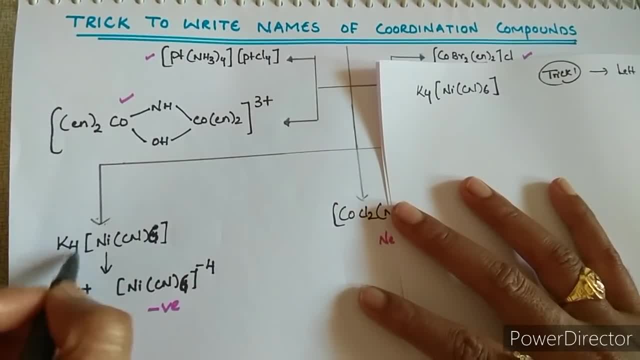 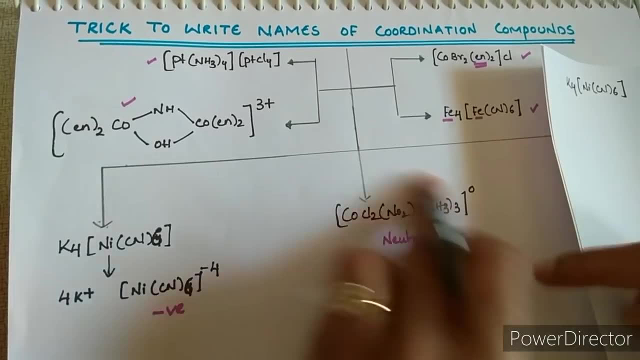 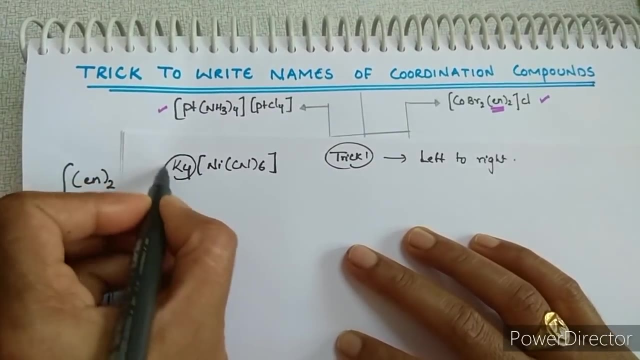 left to right, left to right in the sense outer sphere, ions, you have to name it. ok, if outer sphere is not there, coordination sphere, you have to name it. i will teach you how to name inside the coordination sphere in this first example. in this example, first write potassium, potassium. there is no change in the name of the. 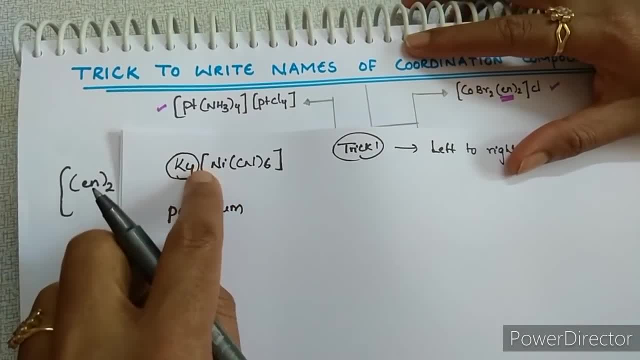 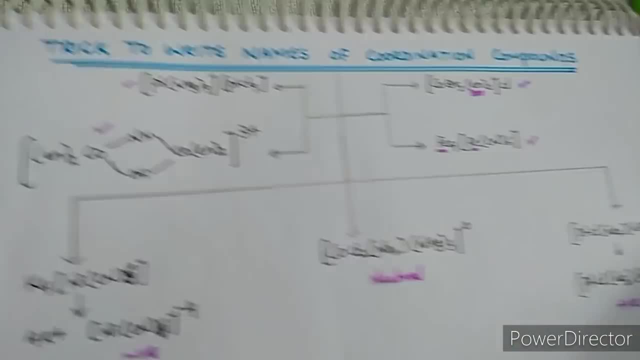 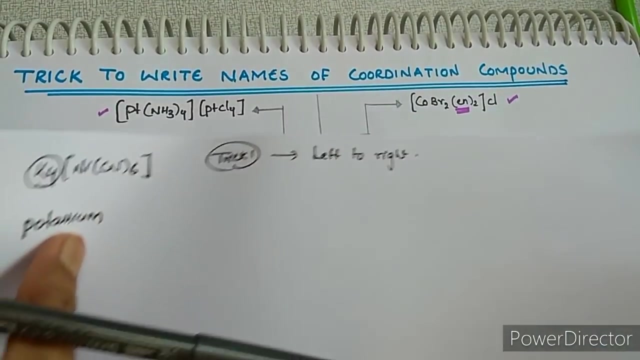 ion which is present as a free ion. this which is there outside the coordination sphere, you have to write as it is, there is no change it. and which is there outside this sulfate also same whatever there inside the sphere, only the axis, only again. for that only we have to do the changes. after that you need to name the coordination. 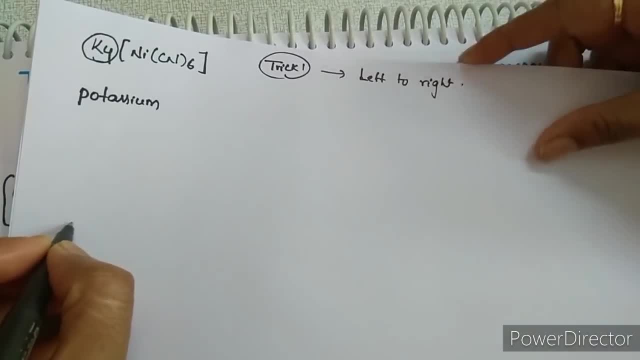 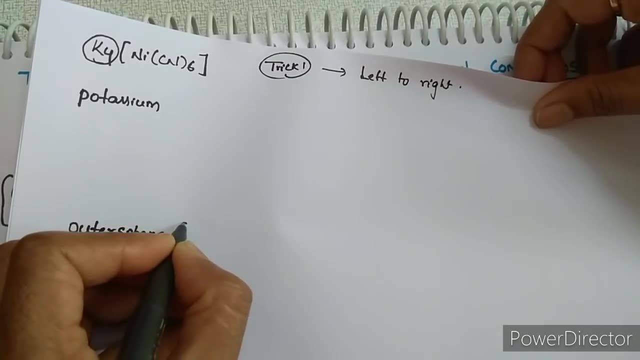 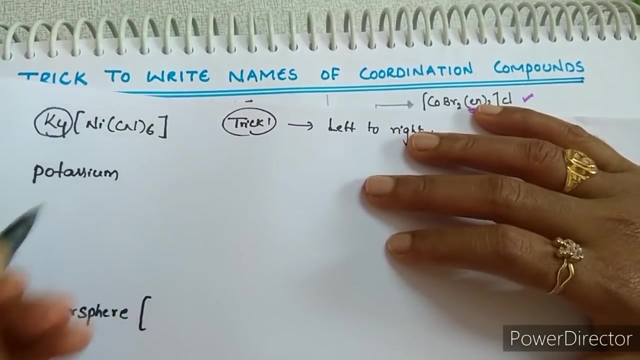 complex. so first what you are naming, you are, you have to name first outer sphere, outer sphere, after outer sphere, what you should name, you should name the coordination complex, open the bracket. then here what you have to means open the bracket in the sense here you should no need to put. 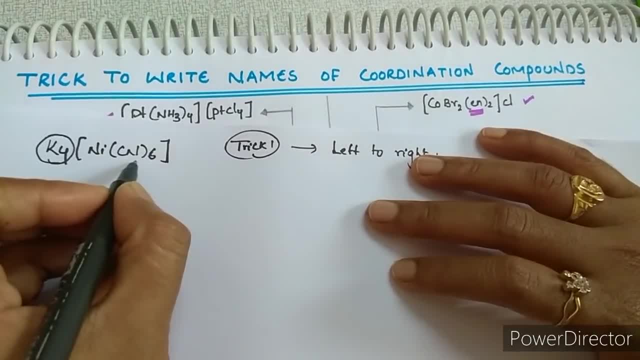 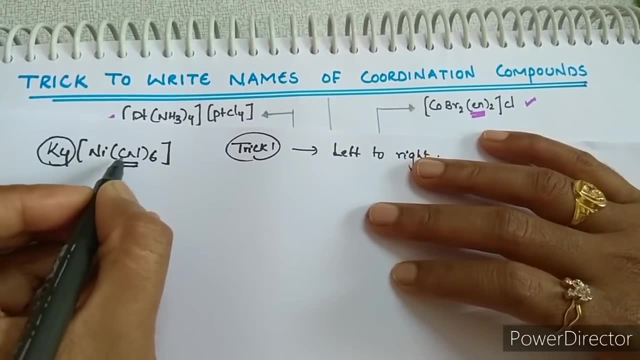 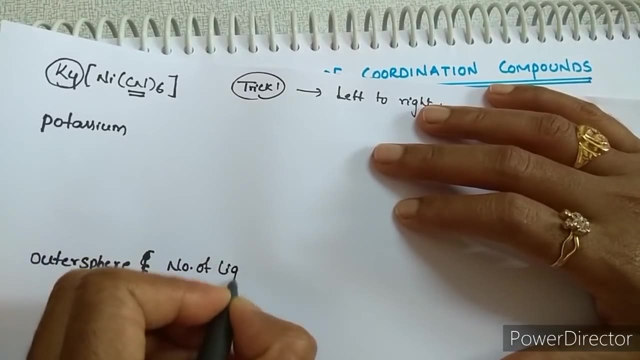 bracket here. bracket is there. that's why i told otherwise, remove it. and here, when you are naming coordination complex, find what is the name of this ligand. just observe it, okay. and how many ligands is there. so what you should do: number of ligands- you have to write number of ligands and name of. 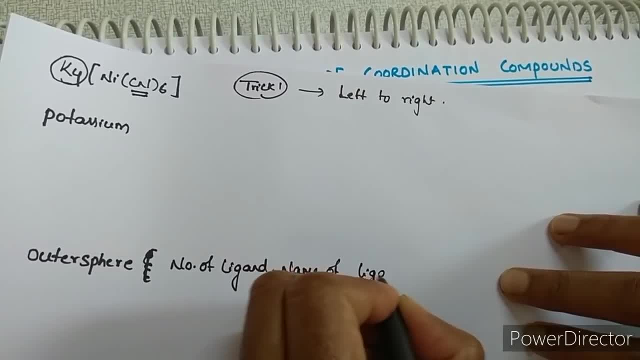 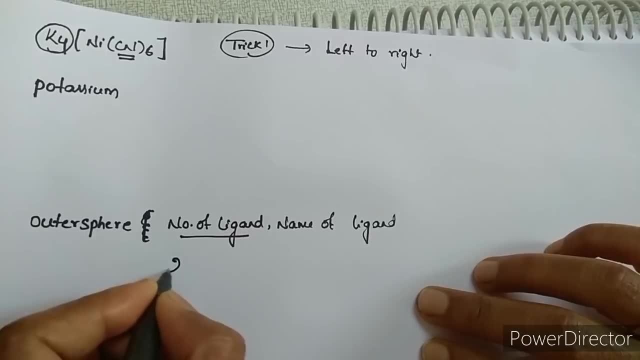 ligand, name of ligand. so after naming outer sphere number of ligand into name of ligand, number of ligands. how to write is: if two ligands is there, you should use a word die. if three is there, you should vote. use a word try. 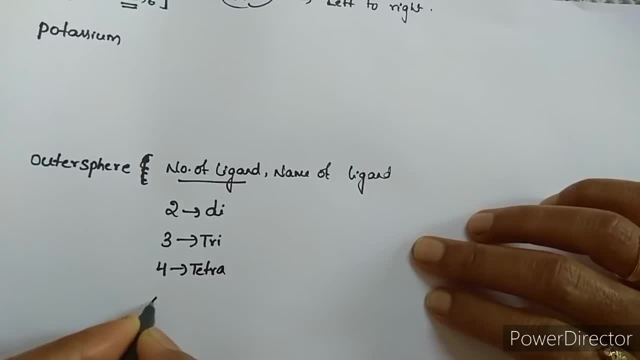 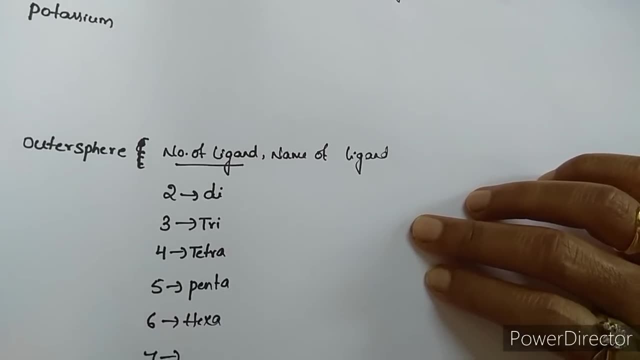 if four is there, you have to use tetra. if five is there, you have to use penta. if six is there, you have to use hexa. if seven is there, you have to use hepta. like that, how many ligands is there? maximum will get two, three, four, five, and also you have to write number of ligands into name of ligand. 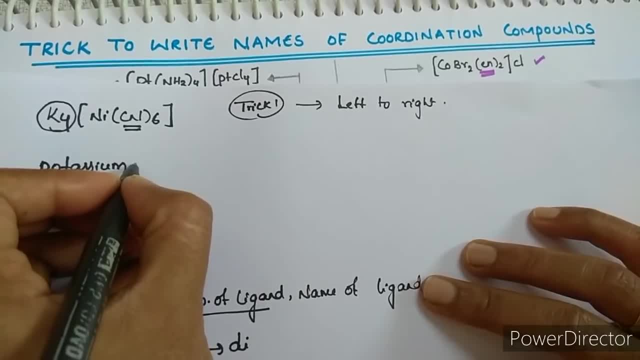 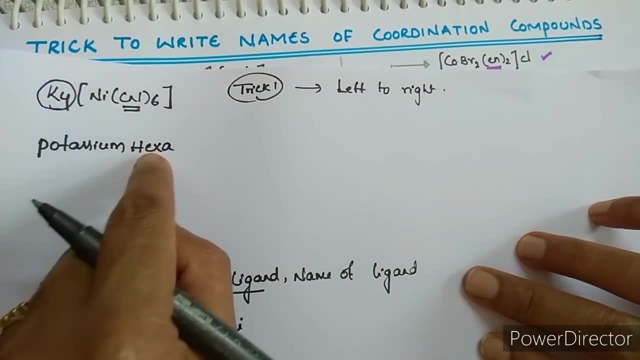 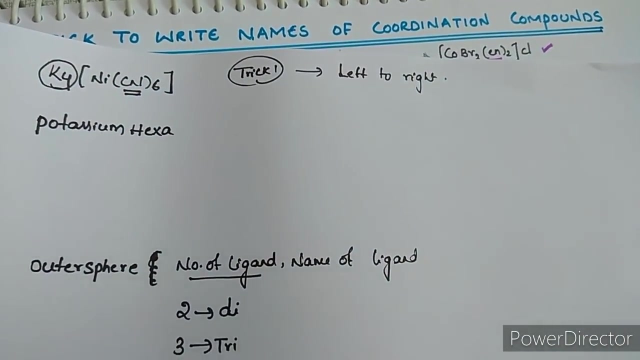 so you can here six ligands is there? so i use the word hexa. okay, you, if you can give gap, little gap, you can give here between this outer sphere and the coordination sphere. hexa, after hexa, cyanide cn is there? ma'am, how you are telling a cyanide? i am going to give you some list of ligands. go through. 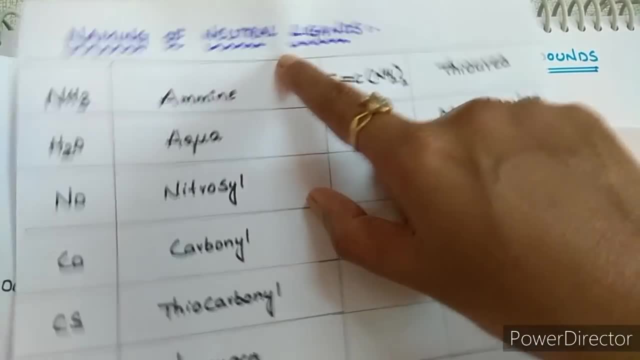 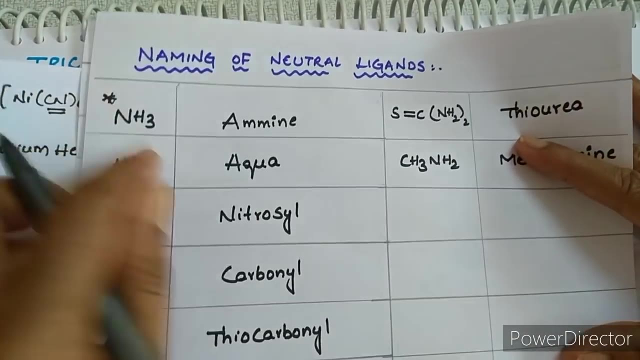 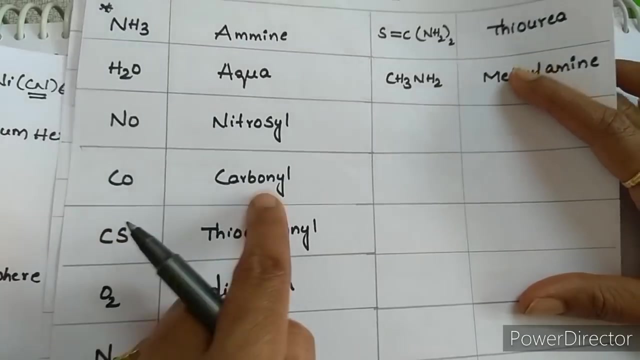 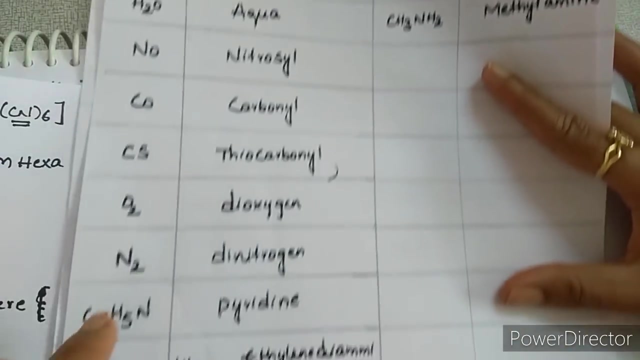 this list and copy it. this is these are neutral ligands. nh3 means amine. one time i will read few these are different from nh3. normally we say ammonia, but here it is amine. h2o, aqua, no nitrosyl, co carbonyl. c is thio carbonyl. up to here these names are different from of ligand names normal. 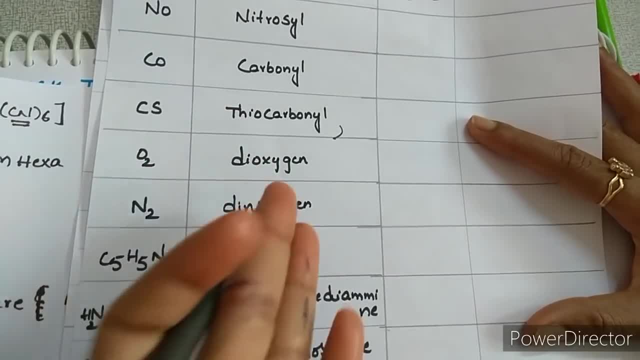 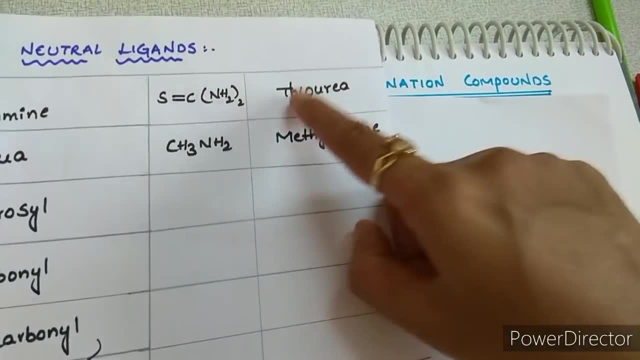 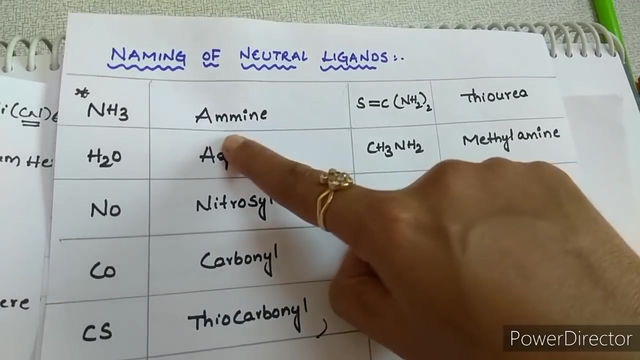 naming from here examples: o2, normally dioxygen and if it acts as a ligand, also dioxygen. there is no change in these names. please copy it, okay. thio urea means thio urea, only amine, methyl amine only when it acts as a ligand. but when nh3 acts as a ligand it will be ammi amine. 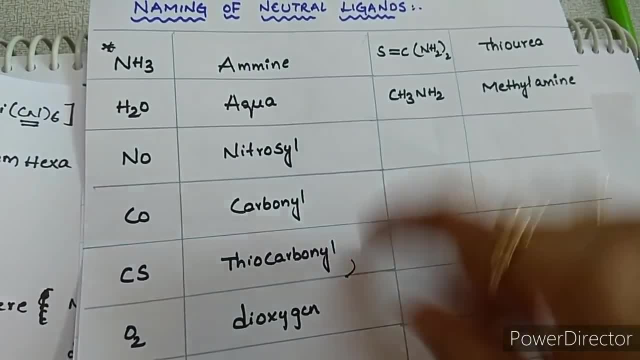 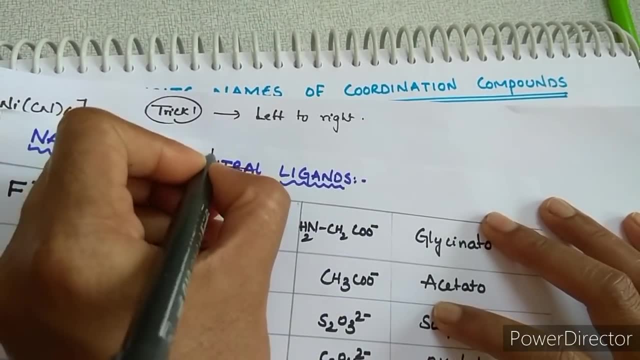 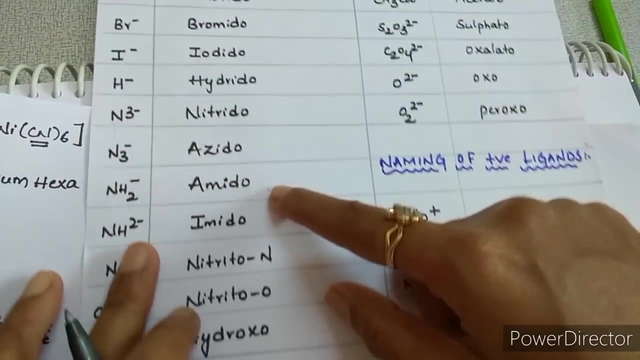 if water acts as ligand, it will be aqua, like that. up to here that there is a change in a name of ligands. observe it. next, coming to the negative, these are negative ligands, negative ligands. these are some names of negative ligands: florido, florido, bromido, iodido, see once. copy all this. 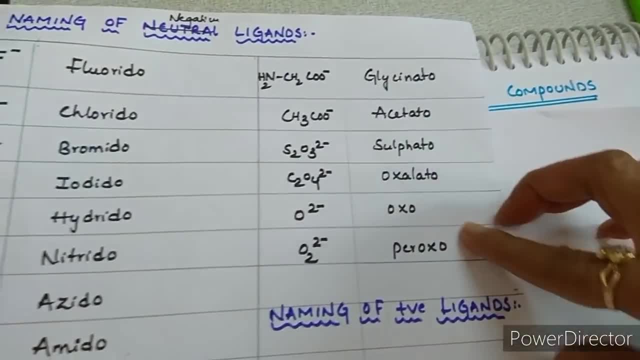 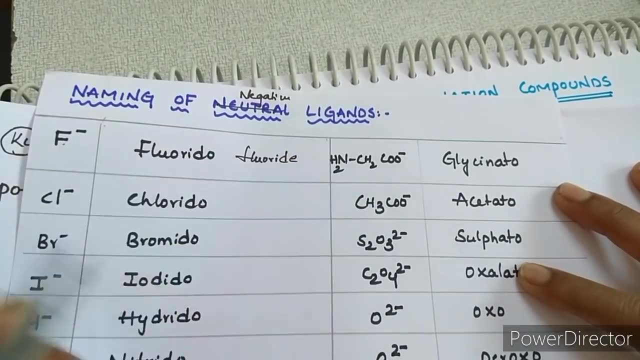 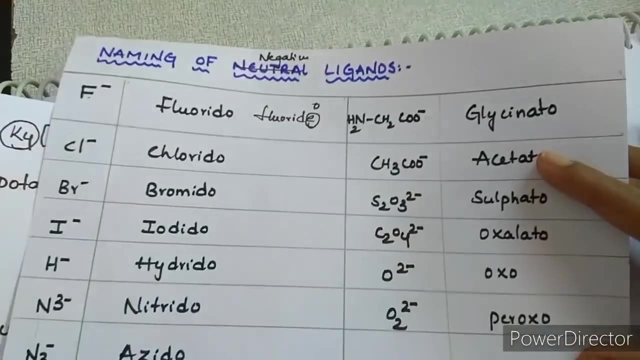 click on pass and copy. okay, these are the ligands. just the simple technique is: this: is what fluoride- no, normally fluoride- you have to remove the e part and you should put o here. that's it. chloride. remove the e part and put o part for negative ligands. this is oxide. remove e part, oxido. you can write: 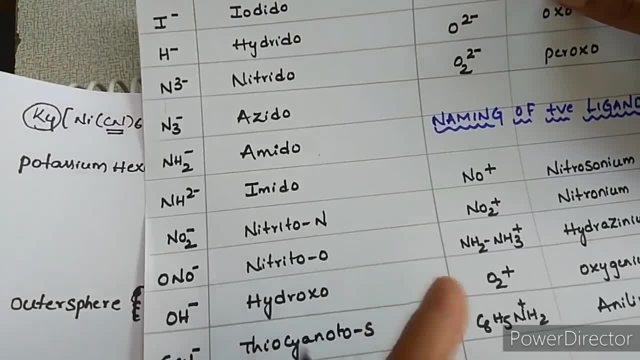 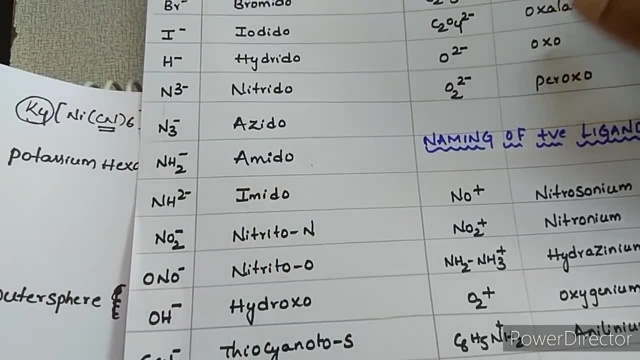 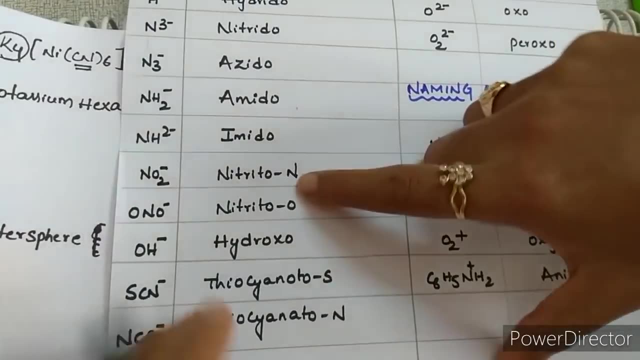 or oxo. you can write okay, like that, wherever this is nitrite, then you can write nitrito, nitrito, MOE and put O. And coming to the ligands which have two donor atoms, those are called as ambidentate ligands, For example NO2. if you absorb nitrogen can donate, oxygen can donate. 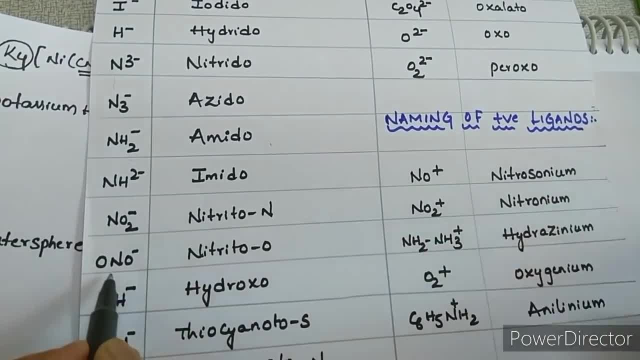 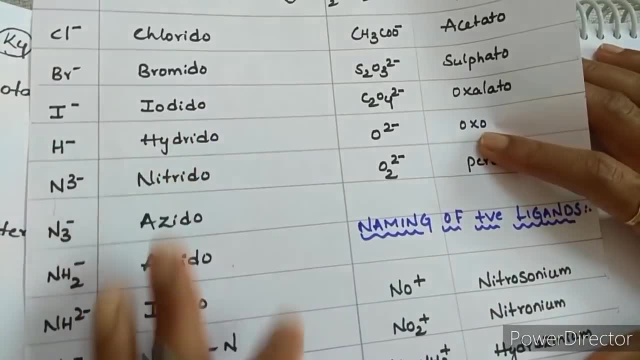 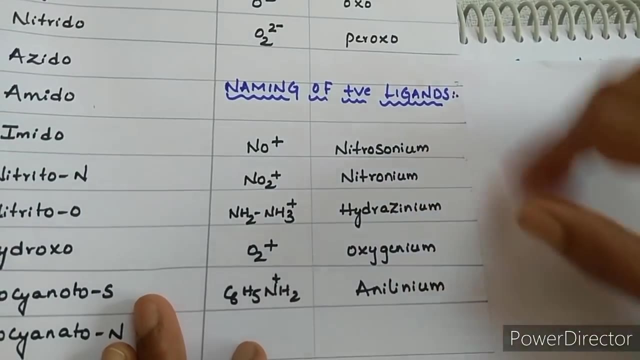 in it. If nitrogen donates, then we say nitrito N, oxygen donates, nitrito O. I will make another session on that. So, based on that, we have to take the ligands, and these are positive ligands. Positive ligands ends with the word IUM, nitrozonium, nitronium, like that. Okay So 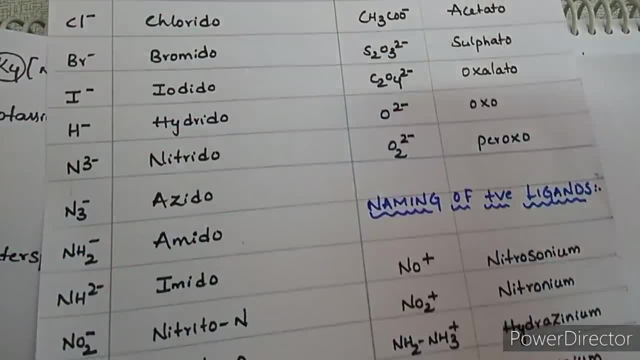 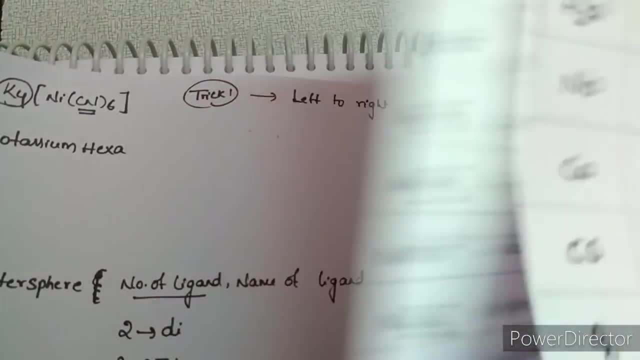 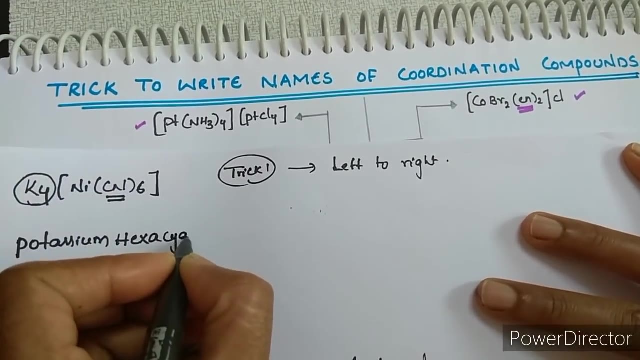 without knowing these names, you cannot write the what coordination compound names, So just copy it and practice these names Now, name of ligand: What CN is there? So CN, what is the name? Cyano or cyanido? Cyanido and carbon is the donor, So 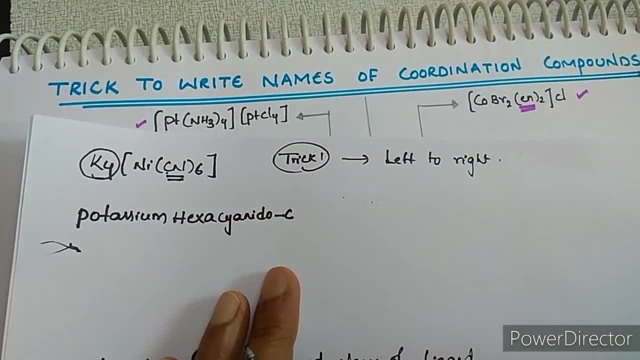 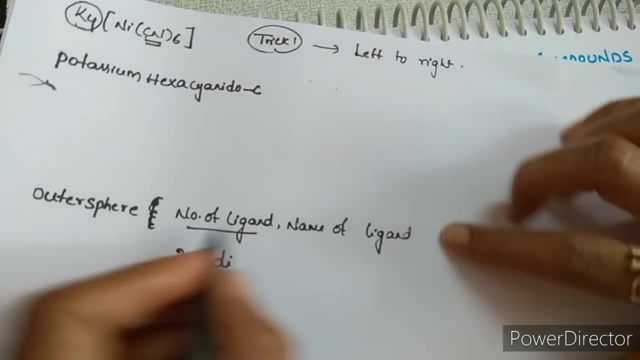 you can write cyanido C Or simply cyanido. Without knowing ligand names. you cannot do anything So mandatory, you have to learn the ligand names. After writing number of ligands and name of ligand, you should write the. 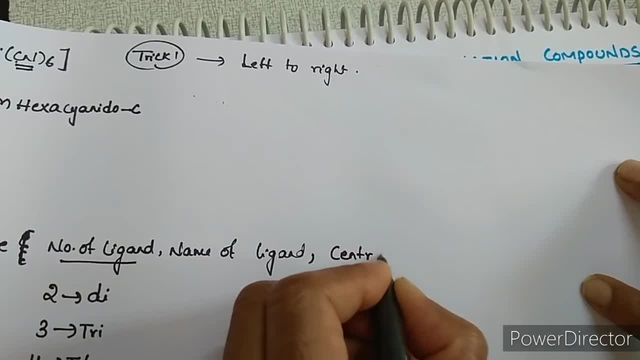 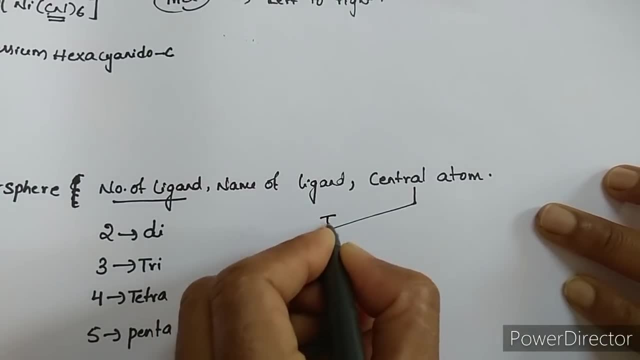 name of central atom. Central atom name you have to write Here. I will tell you simple trick here. What is the trick here? Trick part here is just: you have to observe whether the central atom is present or not. So you have to observe whether the central atom is present or not. So you have to. 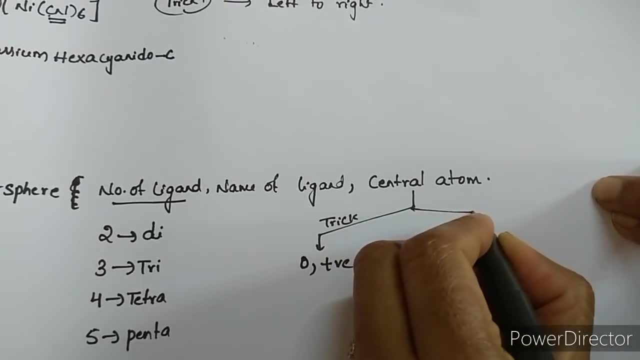 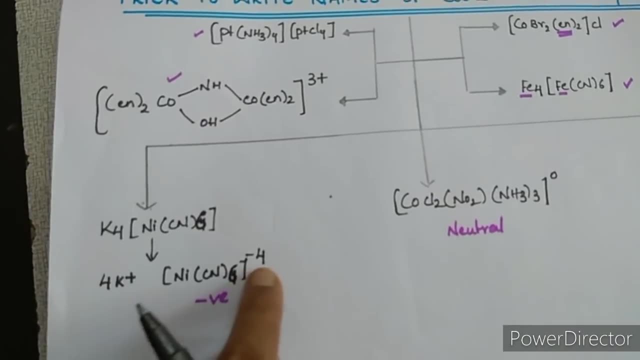 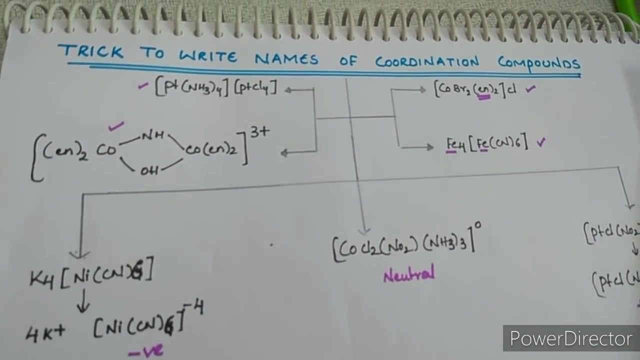 observe whether the central atom is present in neutral ligand, positive ligand, neutral sphere, or positive sphere or negative sphere. For example, as the example we discussed here, the central atom is present in a negative charge, Means the coordination sphere charge is negative. 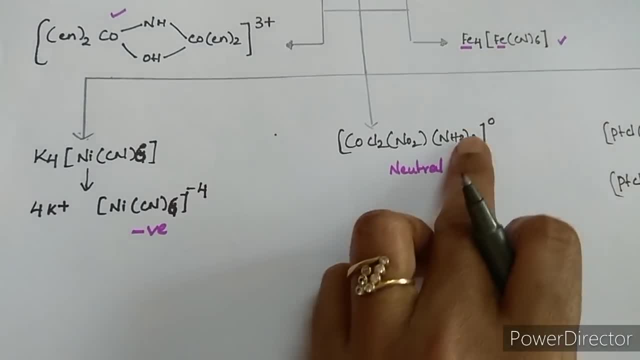 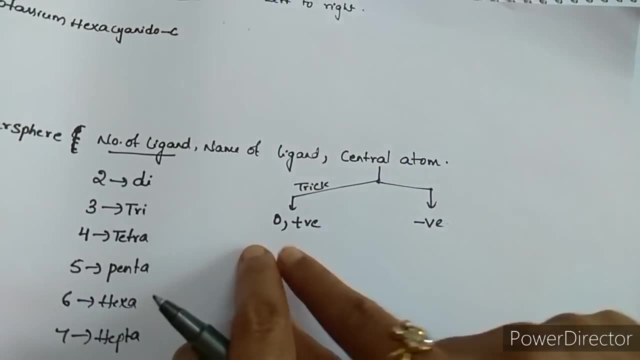 Coordination sphere charge is negative. Okay, Here, coordination sphere charge is neutral. Here, coordination sphere charge is positive. Like this: you need to observe whether the central atom is present or not. So you have to observe whether the central atom is present or not. So you have to. 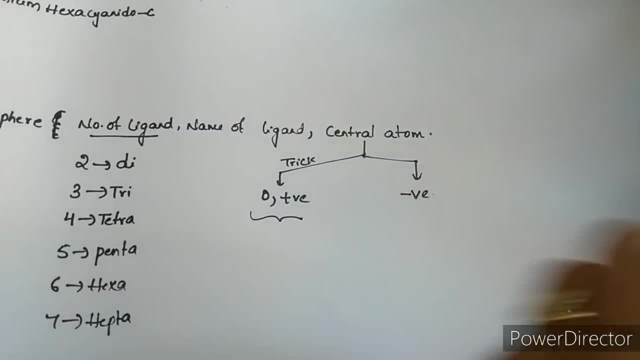 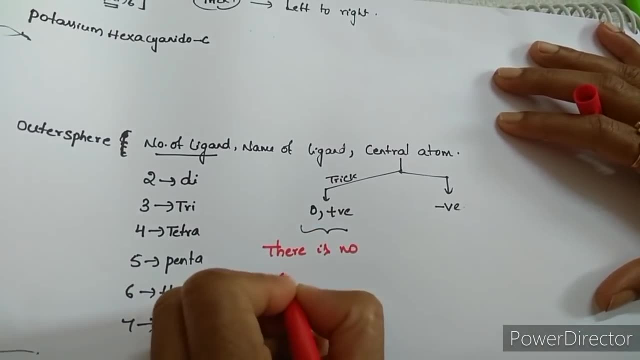 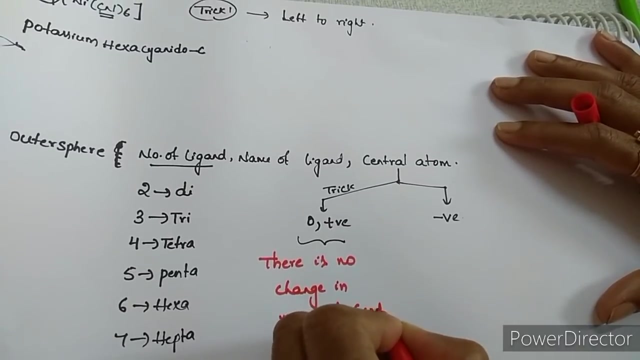 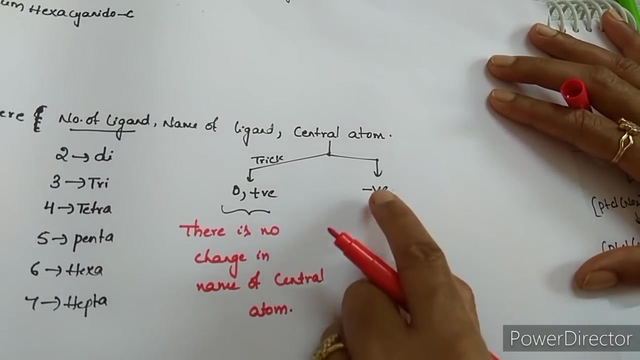 observe whether the central atom is present in neutral, positive or negative. If it is neutral, in positive, then there is no change in name of central atom. There is no change in name of central atom. Clear students, Easy, Just to follow it and practice Definitely you can do Negative charge. 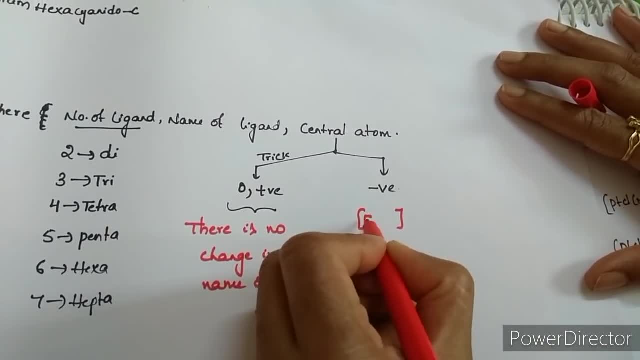 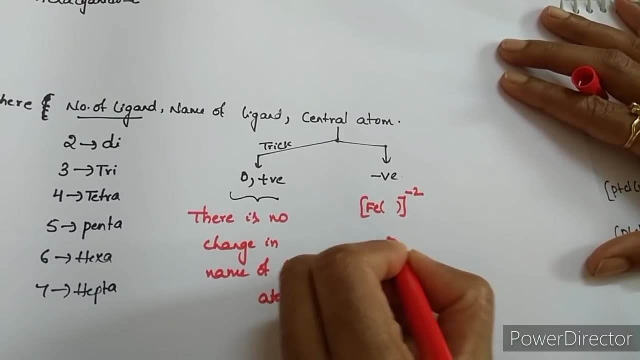 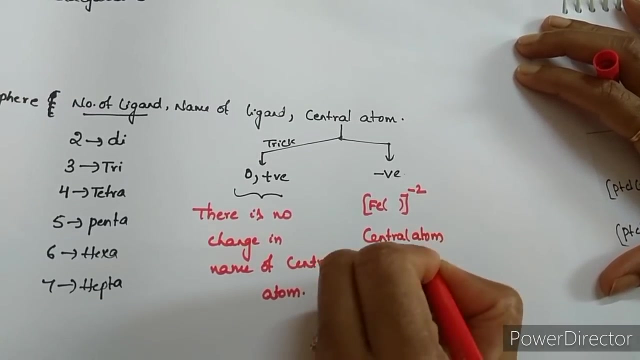 If the central atom is present in a like ion is present, The charge, for example, minus 2 on that particular complex. So this is in this case, you need to end the word of the central atom, Central metal atom. you need to what you should do. You have to end. 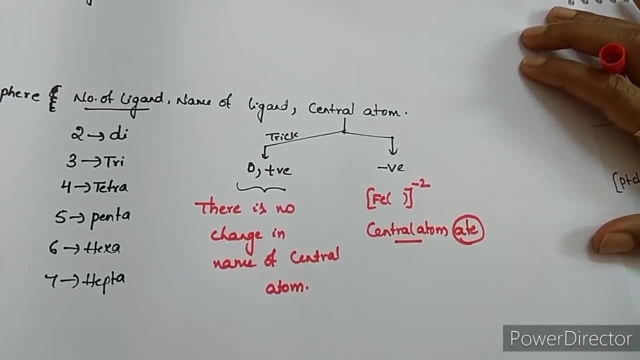 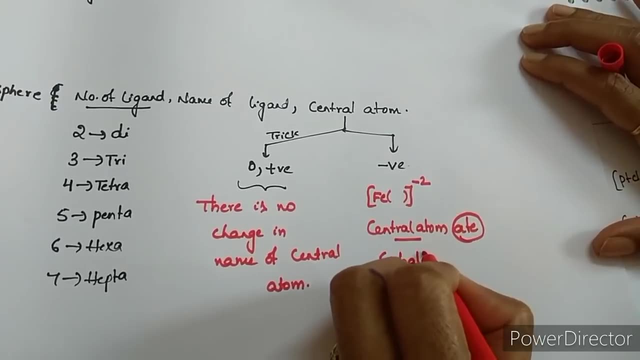 with the word A T E 8.. What to say? A T E 8.. For example, this is cobalt. is there Then cobalt? is there Cobalt? you should write it as cobaltate I? N. in case of I? N, it is. 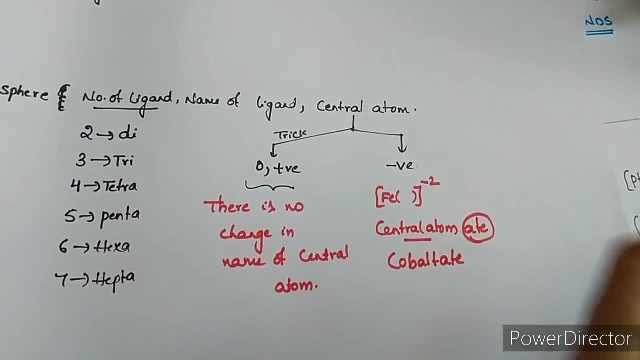 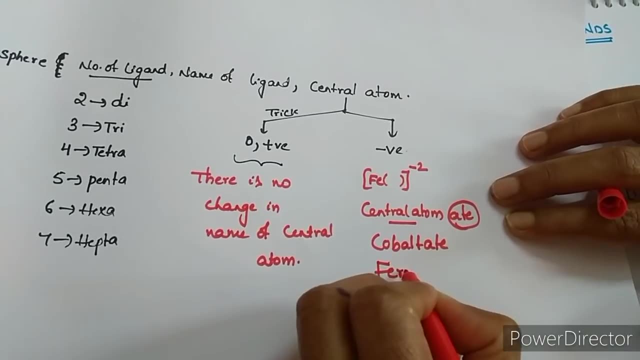 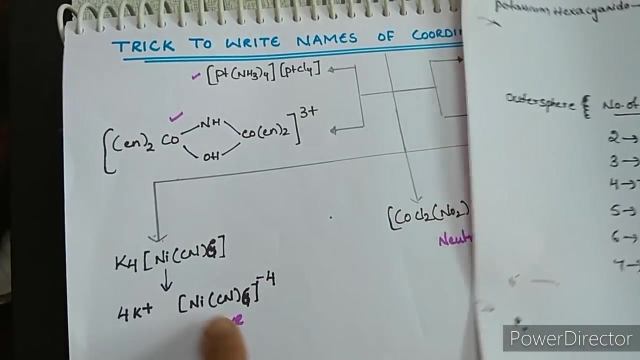 The metal atoms which are derived from Latin names and all You have to write those names, only We will say ferric ferrous, So ferrate, like that we need to write Now. see here: Here nickel is in negative complex, So coordination complex is having negative charge, So whenever it is having 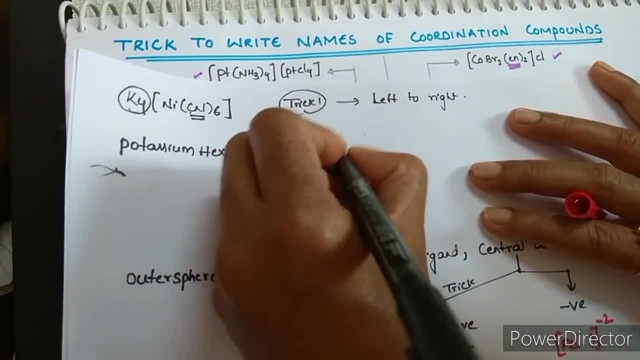 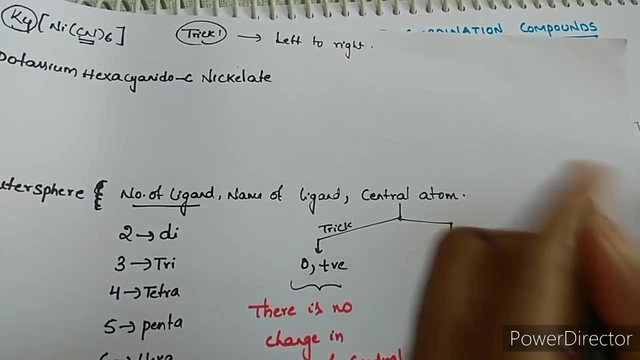 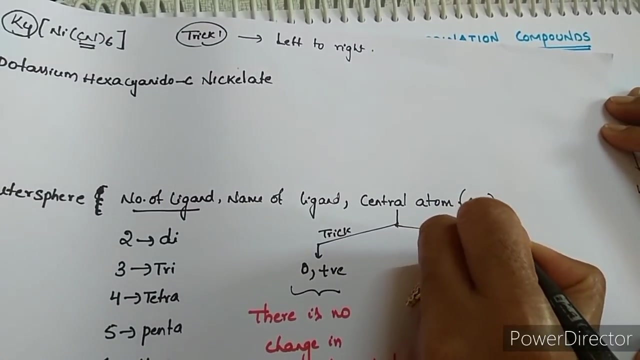 negative charge. what you need to write? You have to write nickelate, Nickel and A T E 8.. You should end with A T E 8.. After central atom, you need to write oxidation state in Roman numbers. In Roman numbers only. you have to write. Okay, Let us see how to find. 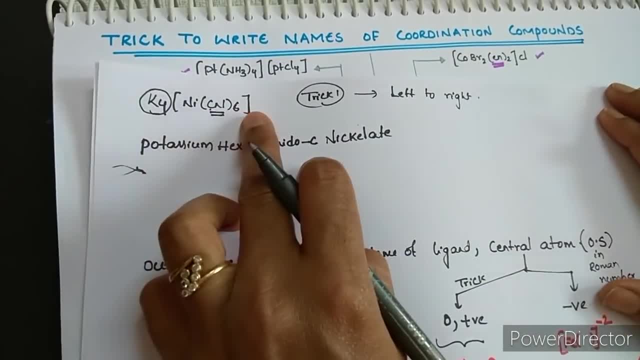 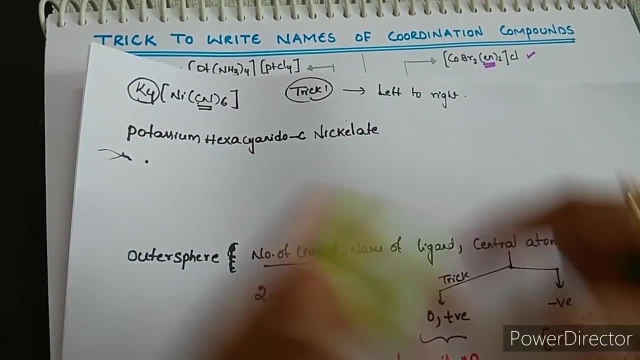 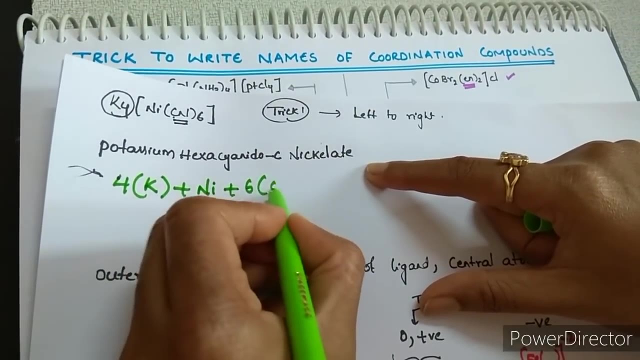 oxidation number for this. The sum of all the oxidation numbers is equal to charge. So how many potassium are there students here? 4 potassium, 4 into potassium plus nickel, Plus 6 into cyanide, which is equal to What is the charge here? No charge, Zero, Okay. 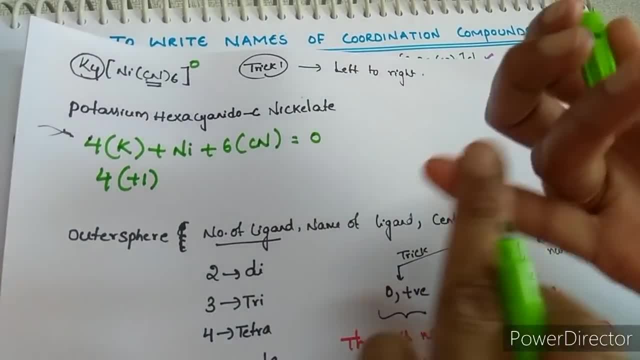 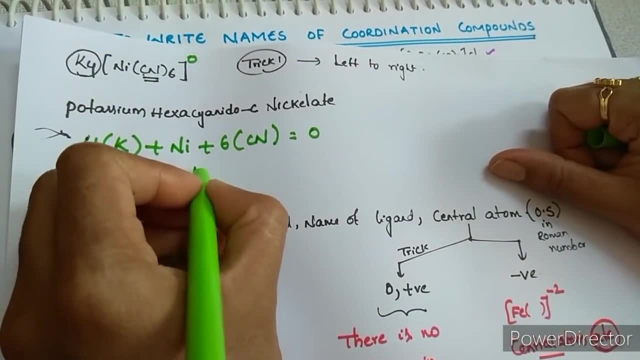 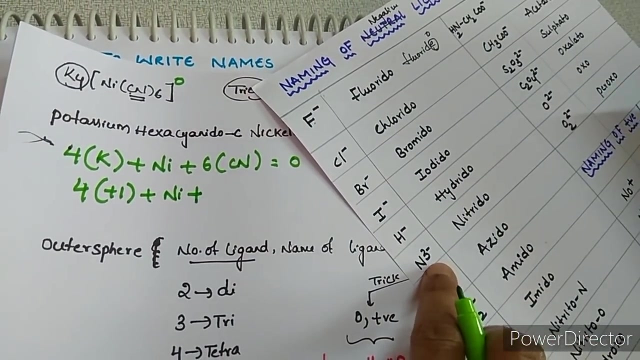 Then potassium is plus 1 because alkali alkali metals- Alkali metals plus 1.. Alkaline earth metals plus 2.. No need to worry for that. And what about a ligand Charge is very, very important. Go through the list and follow for getting the charge on ligand If N is. 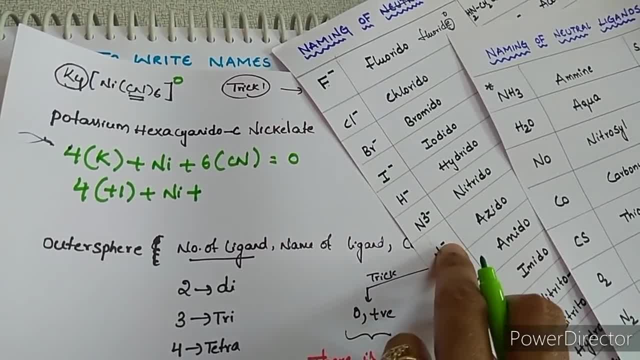 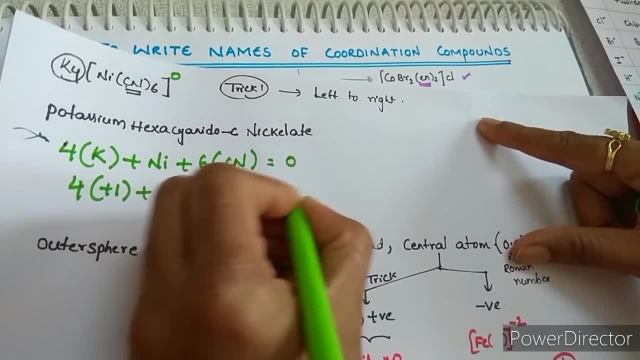 there means you have to take minus 3.. If N 3 is there means you have to take minus 3.. Minus 1. Whatever the charge on there you can take, See N I already gave minus 1 is the charge there, Then this one finding we will get nickel plus 2 state. So nickel plus 2. 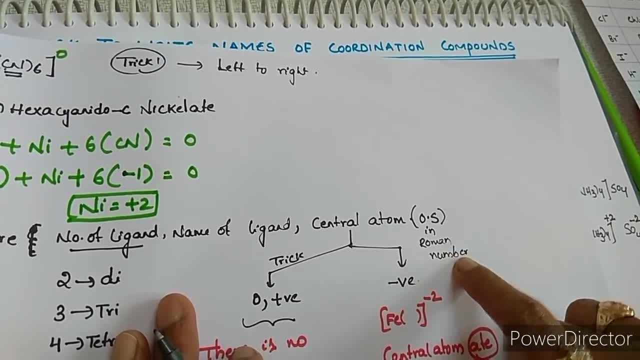 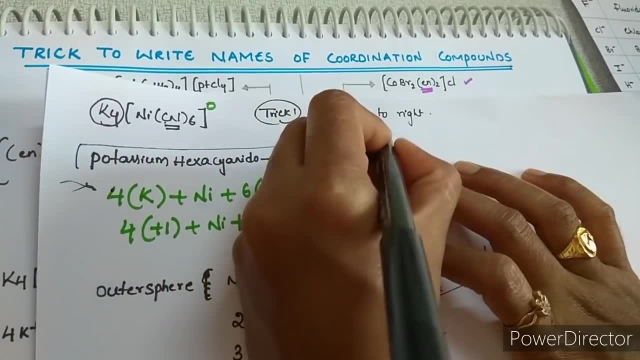 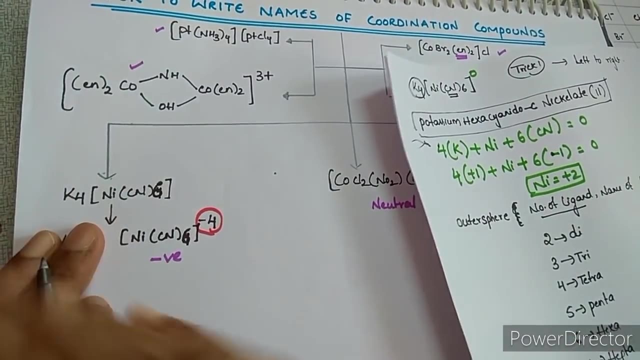 state is there. You need to write in the form of what students Roman number So nickelate 2.. That's it. If here this is in ionic form like this, Like this, For example, this is not given. 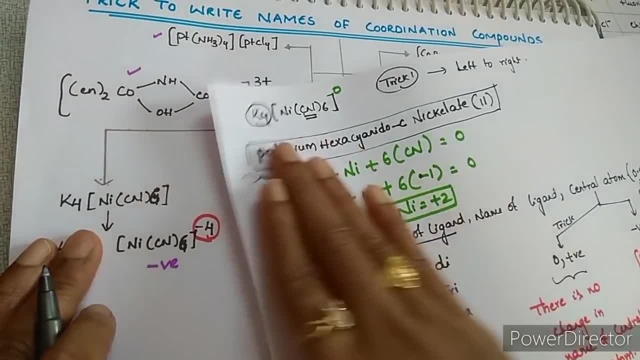 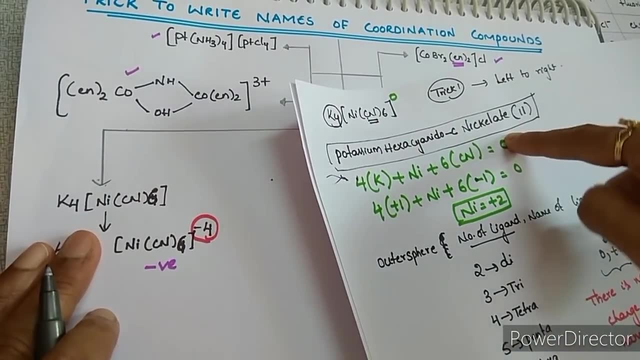 Here this is given in your examination, What you have to do. You won't write 4 K plus here, Just you will write N, I plus 6 C, N, which is equal to what is the charge here Minus 4. you have to write here In those cases. if they give ions in exam, then here you should. 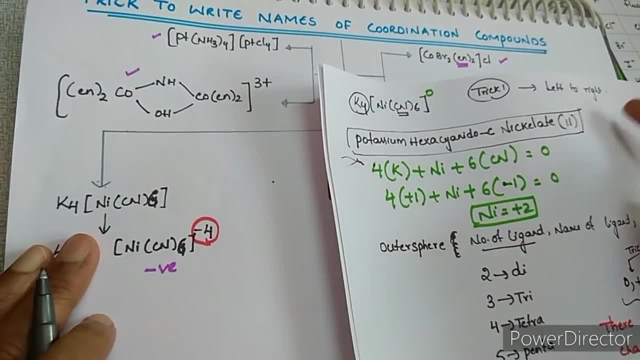 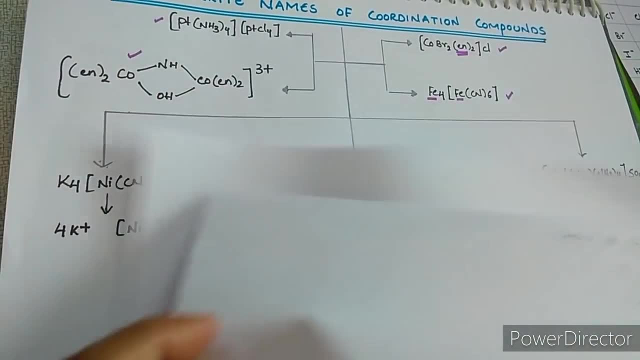 write ion. If there is any negative or a positive charge is there on the top, you have to write ion, That's it. That's it Now. see in a second example how fast you will do now. You will do now. C O. 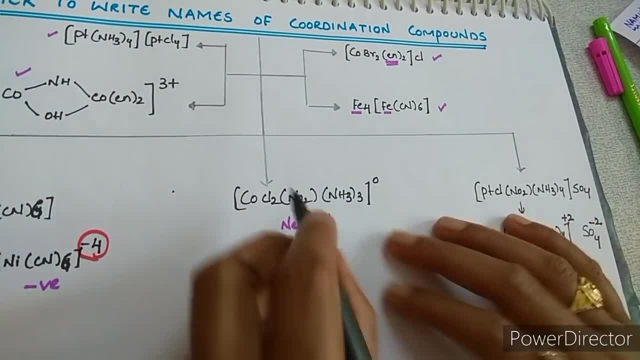 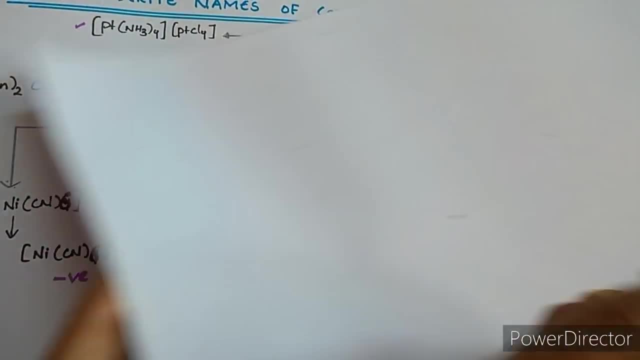 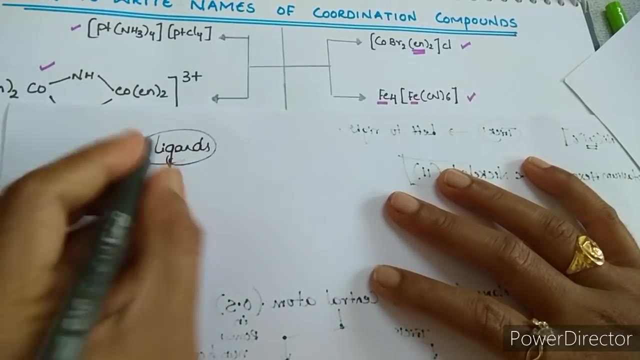 C, O, C, L, 2, N, O, 2, N, H, 3-thrice. So here no outer sphere ions Directly. you have to name the coordination complex, but here different ligands are there. Ya, this point is very, very important. Whenever ligands are there, then different ligands is. 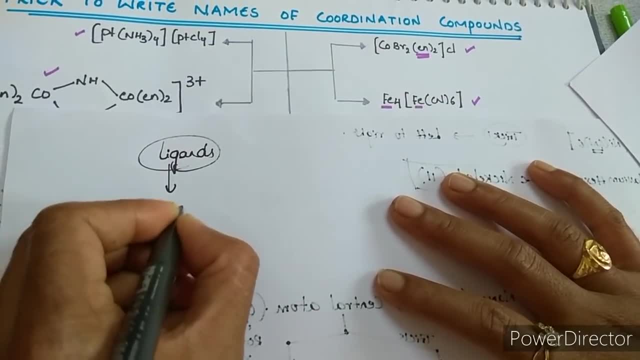 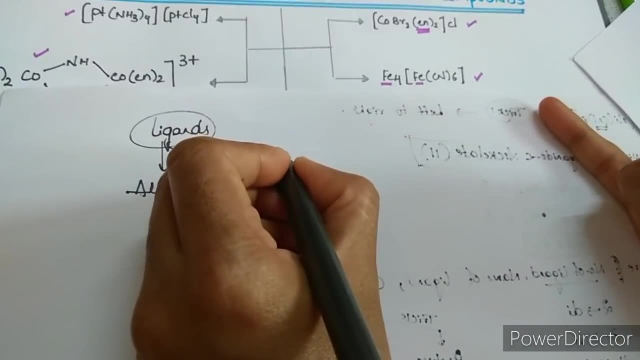 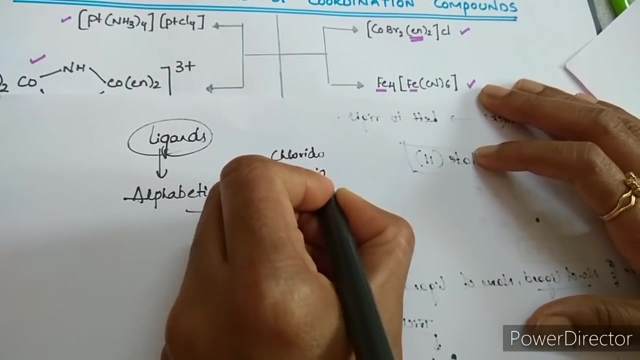 there. You need to follow alphabetical order. You need to follow alphabetical order. like, like, if, if Delpir, IMFROMO, Chloride Chloride Bromear animal, Chloride Bromear animal and bromido, two ligands you are you are having, then b will come first, then c will come first. 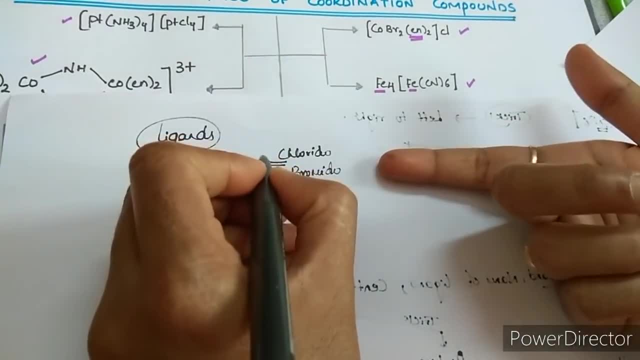 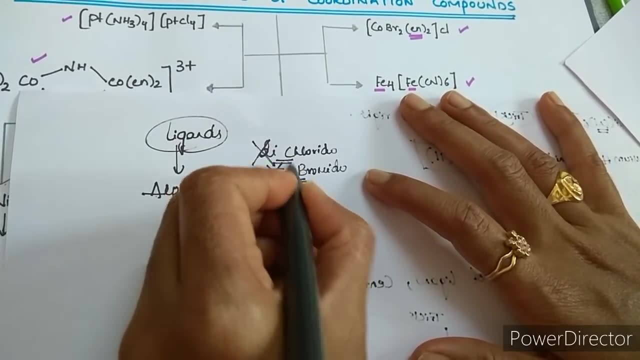 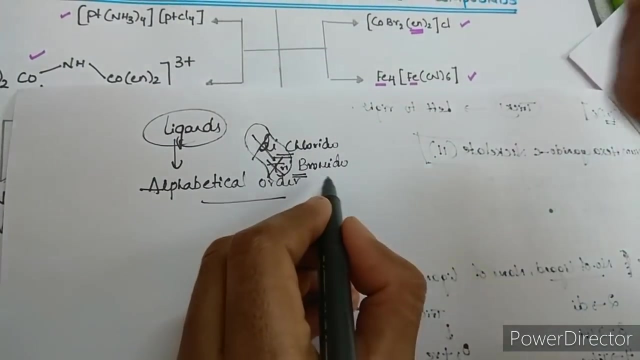 if any two chloride, chloride clins is there, dichlorido, you will write no, you should not consider the prefixes. if tribromido is there, you should not consider these prefixes only, you have to consider the first. what to say? letter of one ligand only. so here here see: cl is what students. 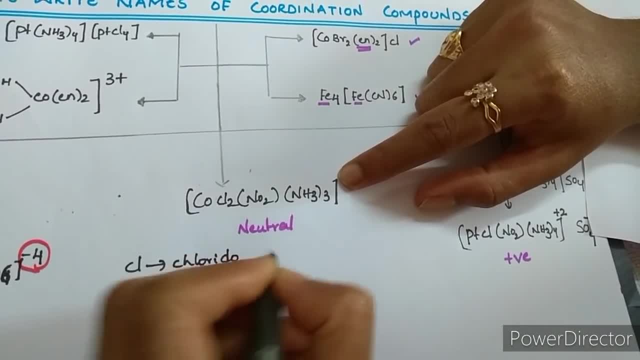 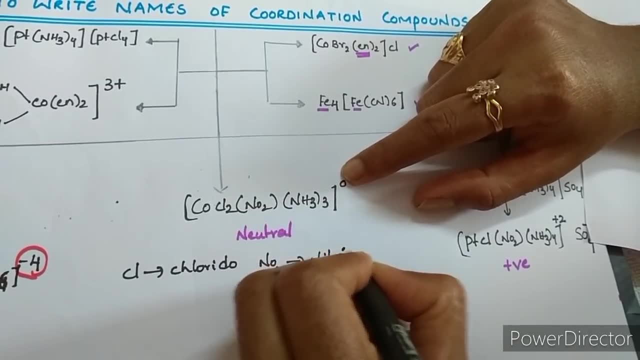 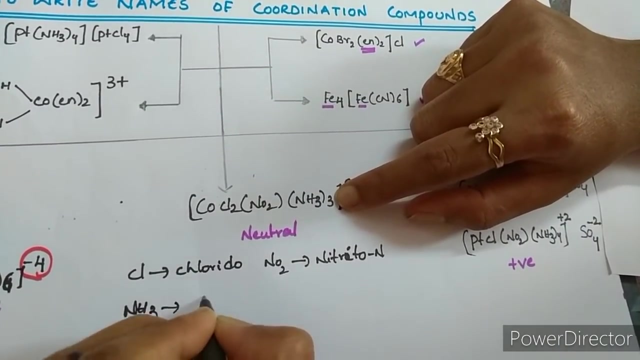 clorido. clorido no2 is nitrito n. you can write, because nitrogen is a donor, which atom come first. that is the donor, nitrito n. if you don't know that, nitro, nitro only, you can write simply nh3. i already gave in the list. what is that? 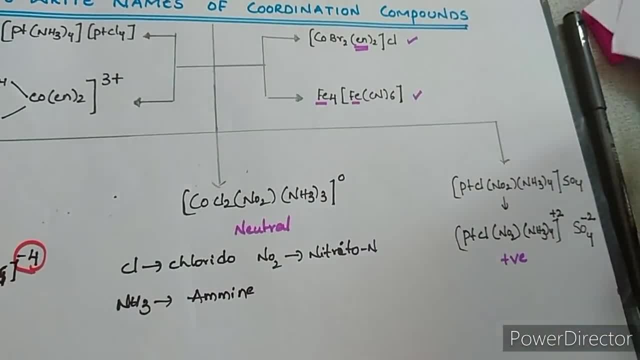 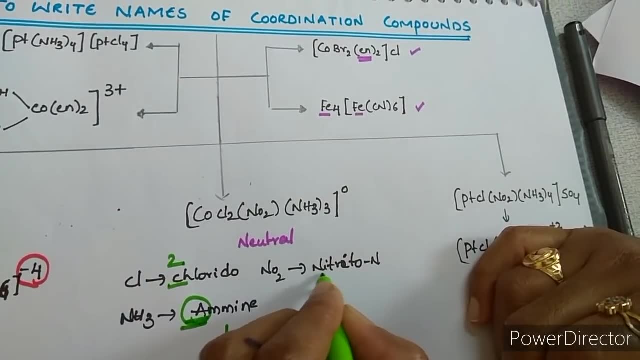 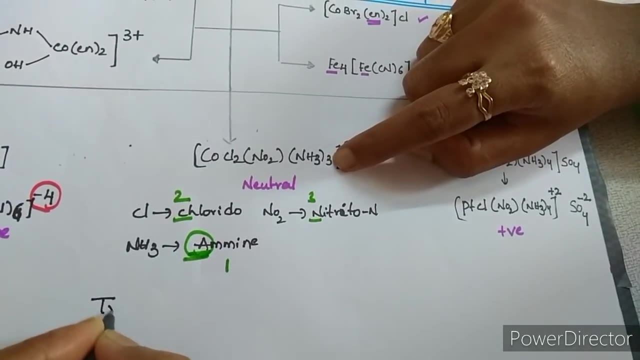 amine, amine. now, as per alphabetical order, which will come first? a comes first, so first priority, next to c comes for second priority. next to this is third priority. that's it. write down now how many amines are there three? three means tri amine, tri amine, here two cloridos are there di. 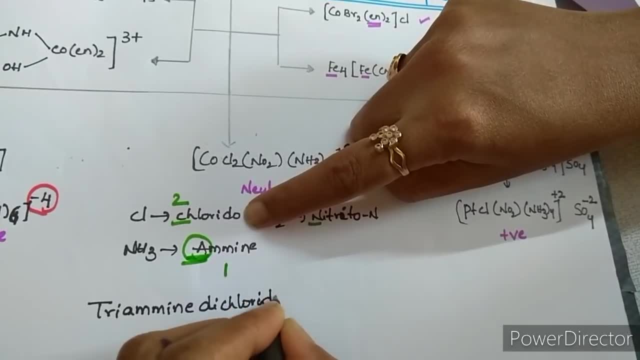 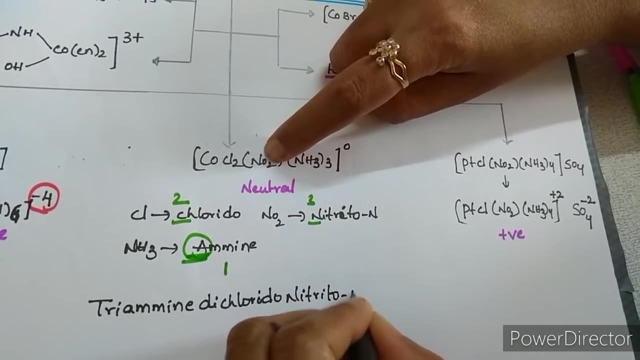 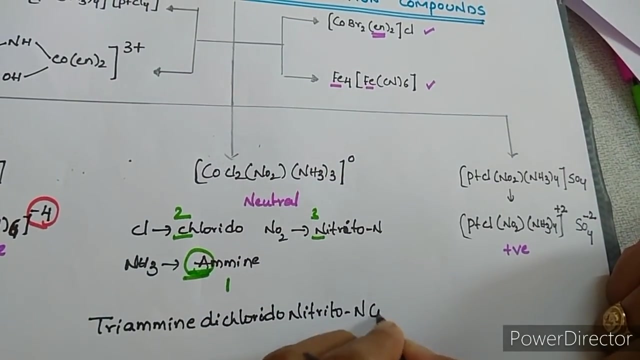 clorido, clorido, and here amine, amine, amine over nitrito. is there nitrito, nitrito, n? all you should write without any gaps. after that write the central atom. central atom charge is zero. so directly you have to write the name only. 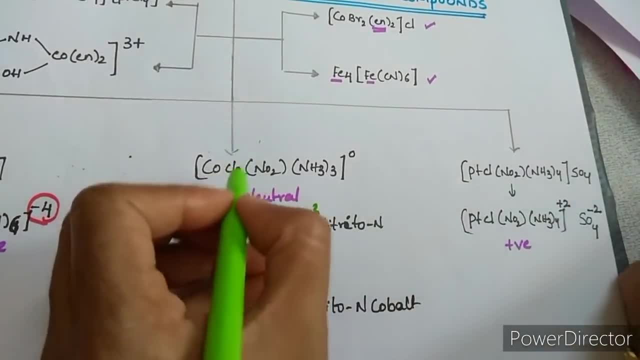 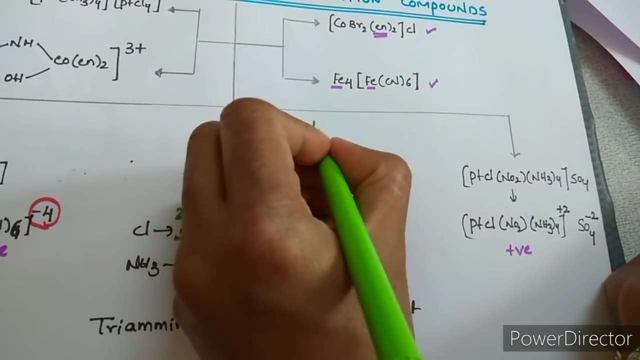 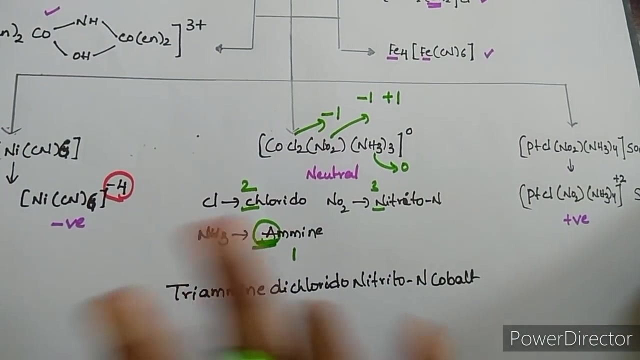 cobalt. and what is the oxidation state? find it, chlorine is minus one, okay, minus one. and no2 is here. it shows both minus one as well as a plus one. that's why i took this example. what you need to consider: ammonia is neutral, no charge on it. neutral again, so you need to take zero. then, if you take here this: 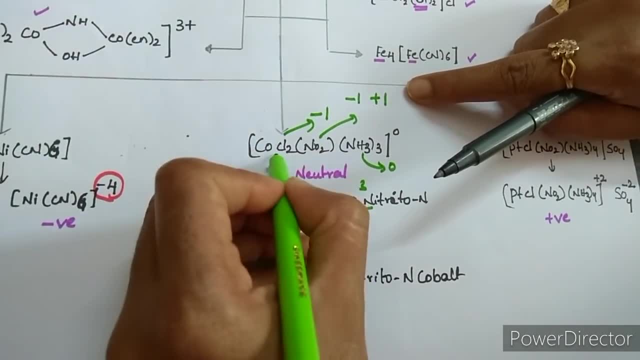 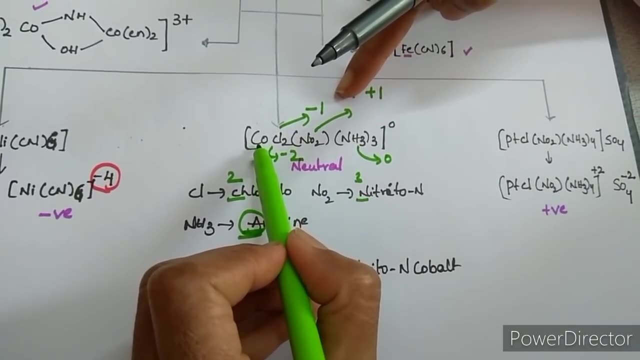 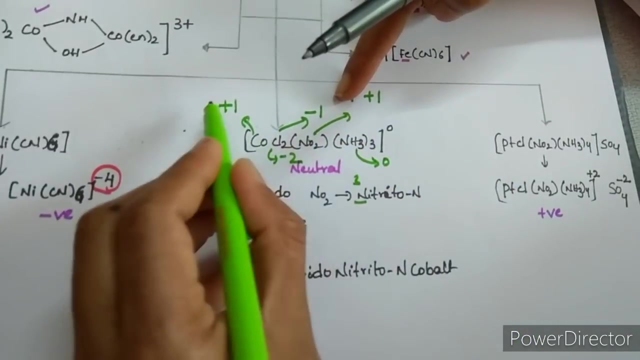 is minus one, then you will get two, are there? so total chlorine charge is minus two, and if you take here plus one for n o two, then the charge on cobalt will become how much plus one? so it won't. it cannot show plus one state. so cobalt cannot show plus one state. that is the reason it. 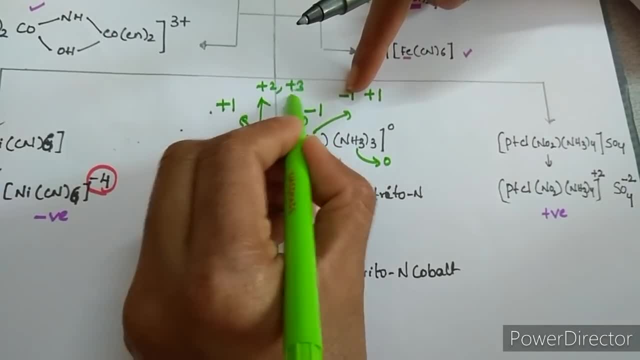 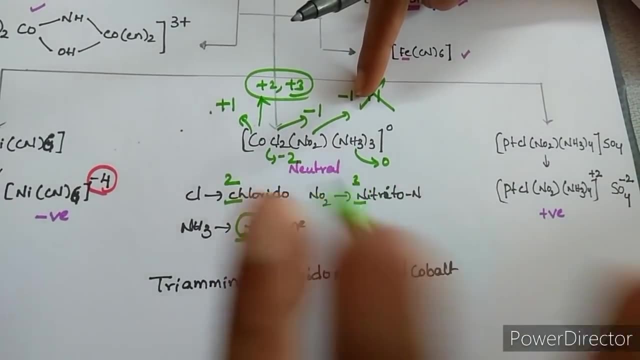 will show only plus two and plus three states. So there is no probability of plus 1 here. That's why you need to take minus 1.. If you take minus 1 here because of 2 chlorines minus 2 and because of NO2 minus 1, total minus 3 will be the charge. 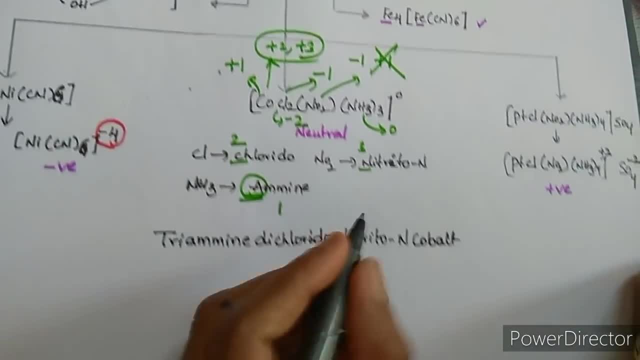 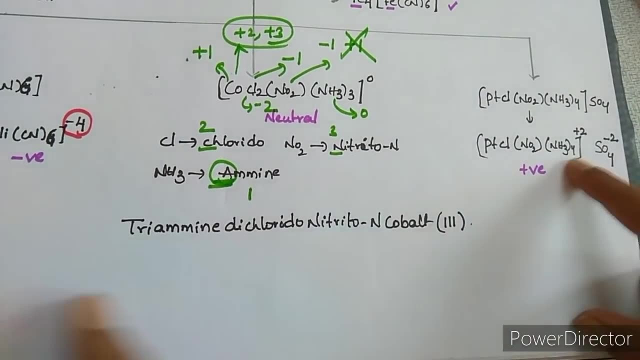 So minus 3, for this means if it goes that side, it will be plus 3.. So that you need to write in brackets like this: Got it? And try this example. This is the homework question I am giving you. 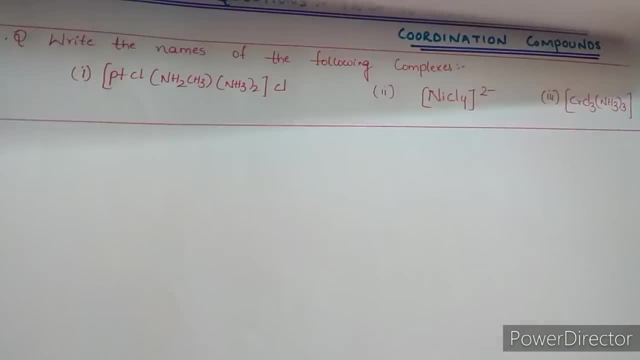 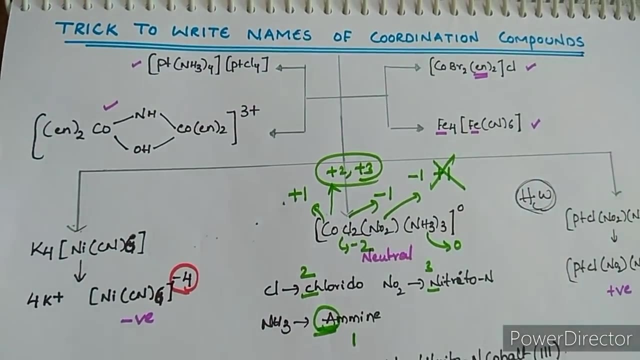 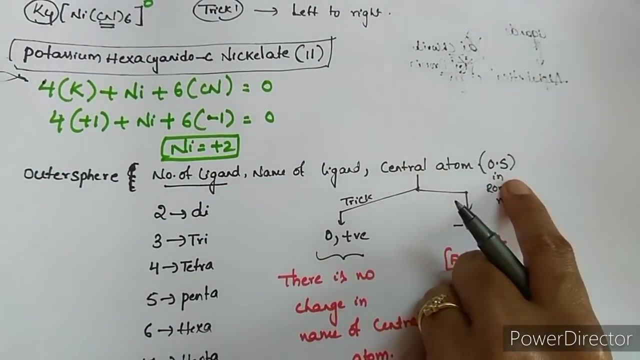 This is the homework question, test yourself question. And this is also test yourself question. Try it. In next video I am going to give the solution to this. What is the summary? students? Outer sphere, number of ligands. name of ligand. central atom and oxidation state. 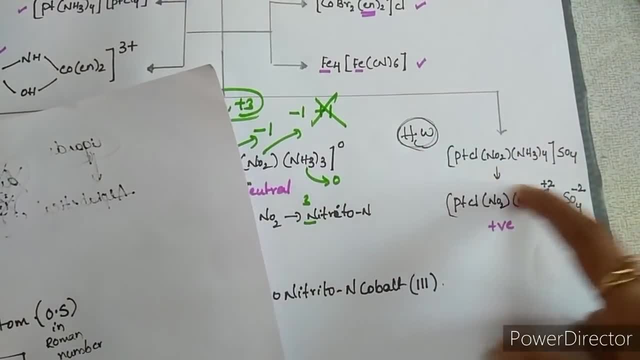 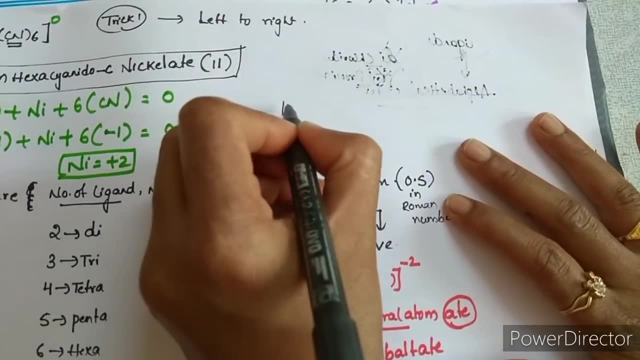 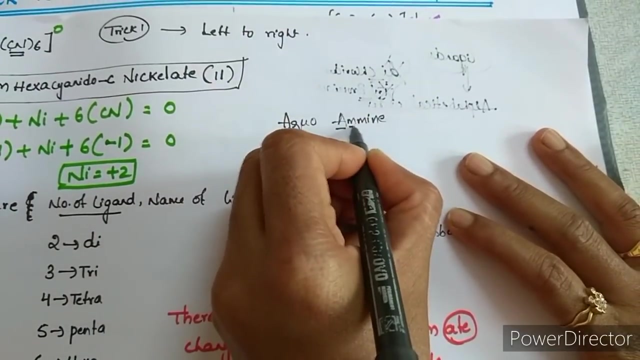 Here, outer sphere is after writing coordination sphere only. you have to write outer sphere, For example. one more point: If two ligands are there which starts with same alphabetical order, like AQUA and ME, Then first letter is same. then you should see based on second letter. 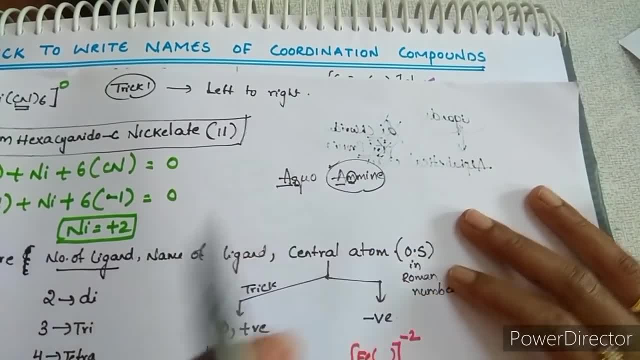 M comes first before Q, So M mean you need to give more priority than the AQUA. I thank you so much for watching. My name is Komali. I am your chemistry mentor.